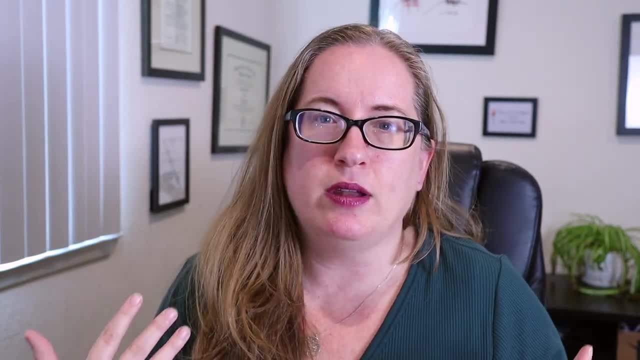 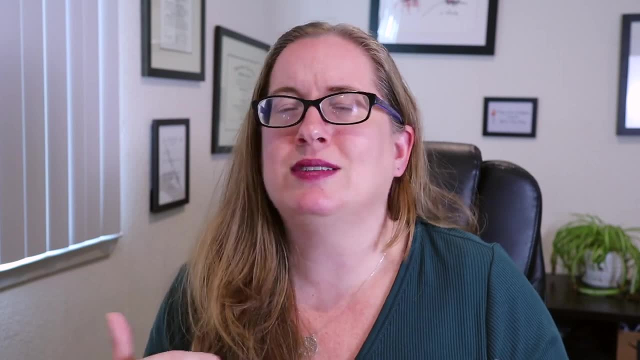 companies that I would do anytime. I would ever hire someone to help me with anything in my business And I'll show you the kinds of things I look for to figure out if a business is sketchy or someone I should actually be doing business with. So let's get started. 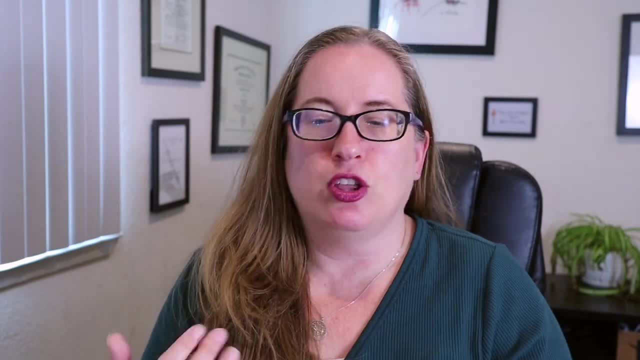 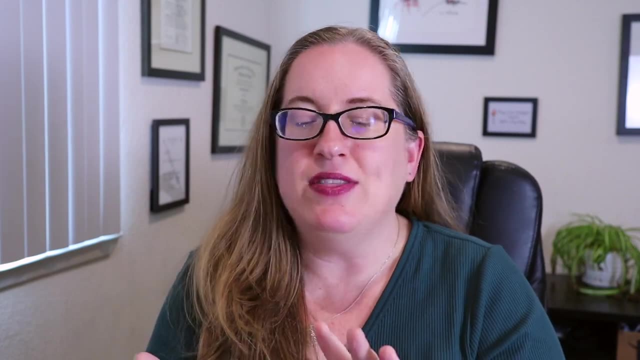 So I picked these four because two of them- Trademark Engine and Trademark Paramount- advertise a lot on YouTube and I see them here. And then LegalZoom, I think, is one of the big ones that everyone's probably heard of, because they do so many different kinds of things Trademarkia is. 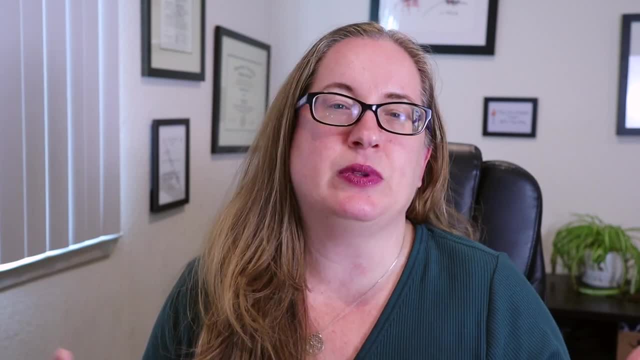 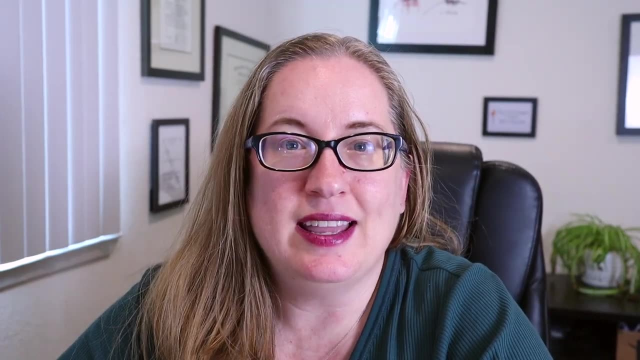 also a big one for doing trademark applications and is a place you can also do free trademark searches. So let's start looking at each of these businesses. So the first we're going to look at is Trademark Engine. Okay, so Trademark Engine is a business that I've been doing for a long time. And I've been doing a lot of business with. So I picked these four because two of them, Trademark Engine and Trademark Paramount, advertise a lot on YouTube and I see them here, And then LegalZoom, I think, is one of the big ones that 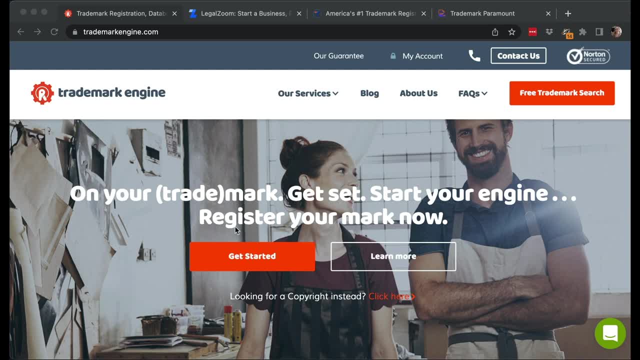 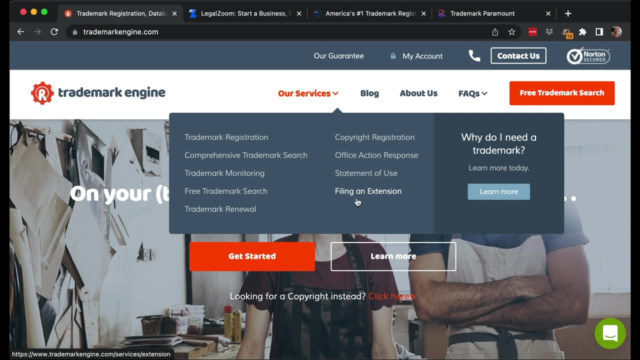 Trademark Engine. Okay so, Trademark Engine. Okay so, Trademark Engine. They have a website here. looks like a fairly nice, normal website. it looks like they actually do multiple other things. They do trademark stuff And they also do copyright stuff, And then they you can get them to help you with. 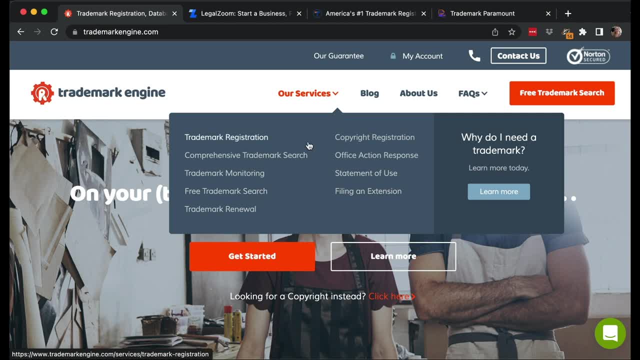 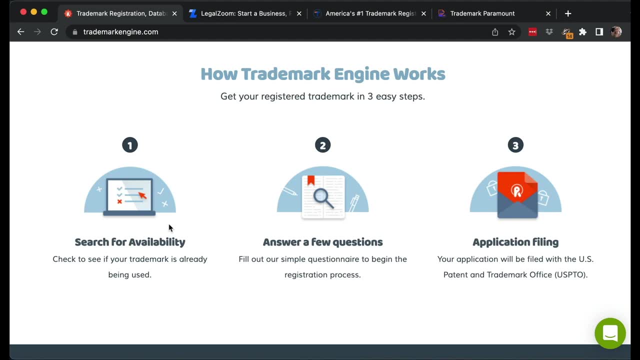 multiple different types of things for a trademark, including registering your trademark, responding to an office action, etc. So let's first just look at if you want to just register your trademark. So they have three different packages that they are offering here. One is doing a trademark search. 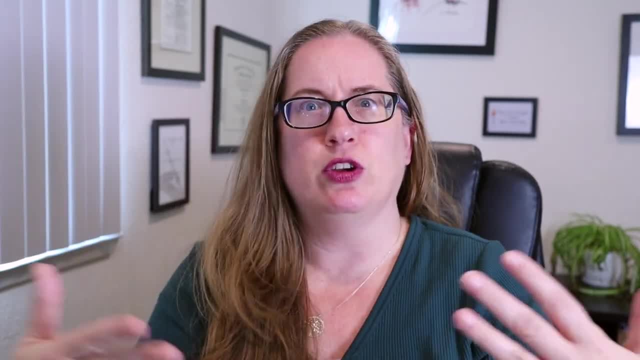 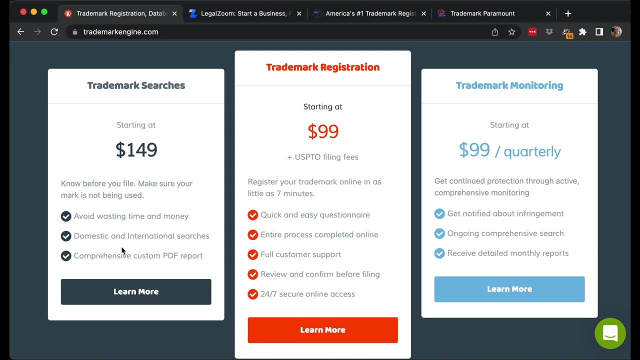 you may want to do a trademark search before you file your trademark. We definitely want to do one on your own, at least searching online in the trademark database. you might want to pay someone else to do that for you. Trademark registration is the actual. 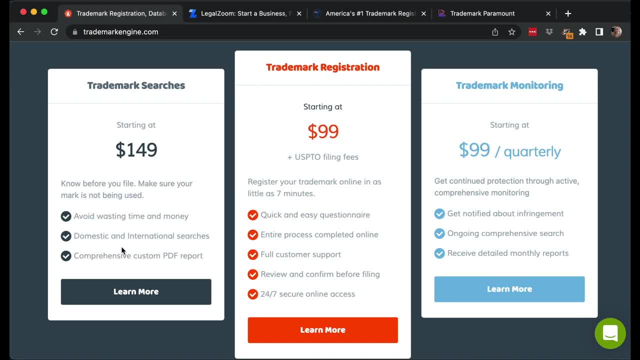 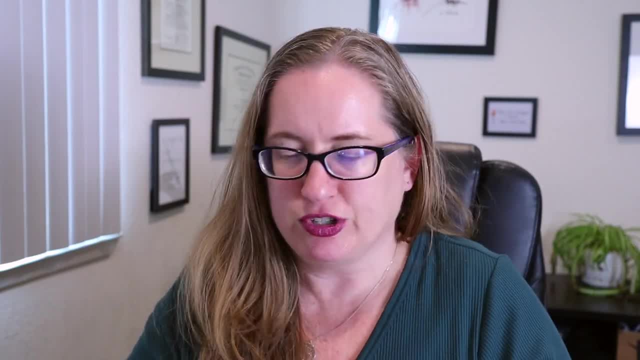 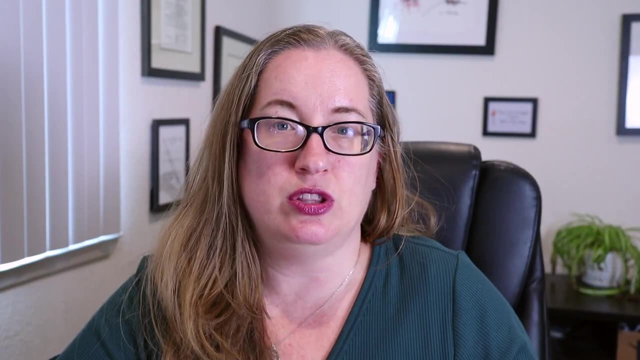 preparing the application and filing it. Trademark monitoring is something where they will theoretically do searches for you and notify you if anyone's infringing, at least by doing online searches. So we're going to look here at trademark registration. it says starting at $99.. And that's not including the the trademark offices filing fees. That's normal. I would not say it shouldn't include the term of filing fees because it depends on how many classes you're filing in. Typically you're either going to be $250 per class or 350 per class, depending upon how you do your application. So it says you can register. 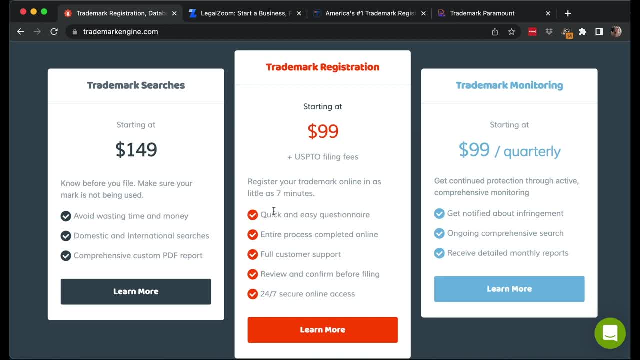 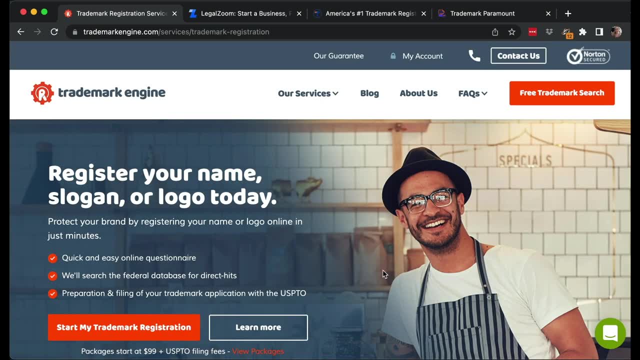 it as little as seven minutes, which seems strange, but quite as a questionnaire, the process: online customer support, online access. okay, we're gonna hit learn more. to learn more about this, we're going to the specific website. let's view the packages and see what kind of packages are. 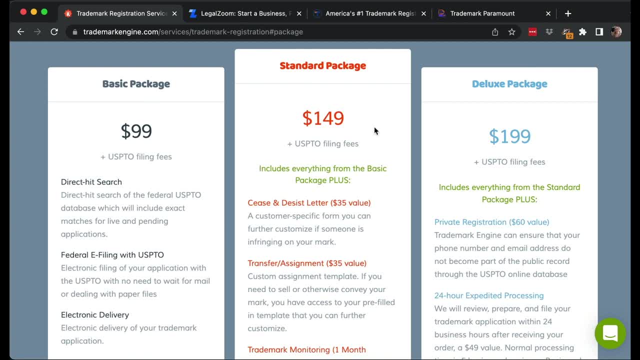 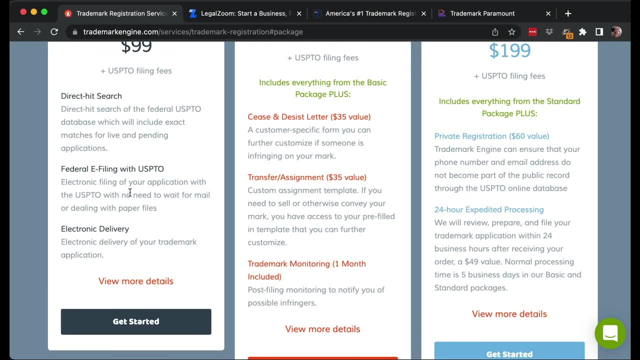 offered. Okay, so the basic package is 99.. Standard is 149.. Deluxe is 199.. Basic package: they do a direct hit search in the trademark offices database. they do the filing electronically, which I would hope they would like please. you're not allowed to do it by paper and 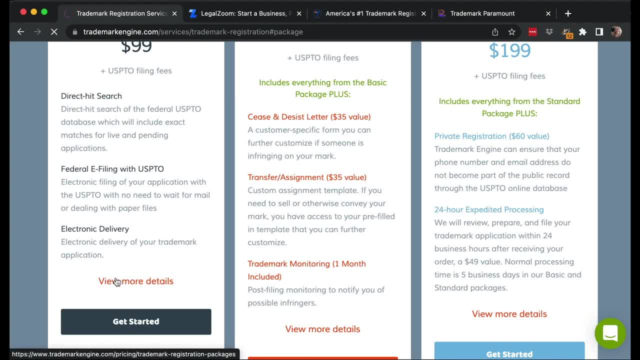 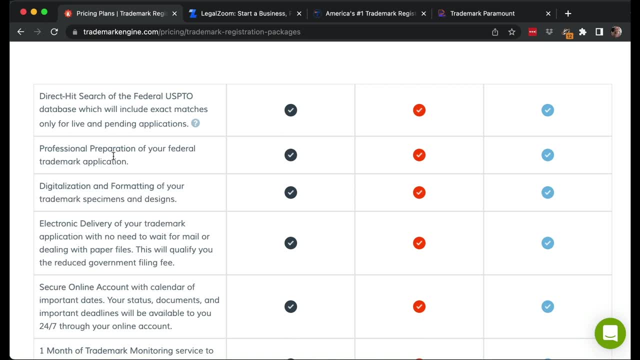 electronic delivery. Let's view more details about this. Is it doing it? Okay, this actually opens up a thing with had a lot more checkmarks, Okay, So direct hit search preparation doesn't say lawyer, preparation just says professional. I don't actually know what that. 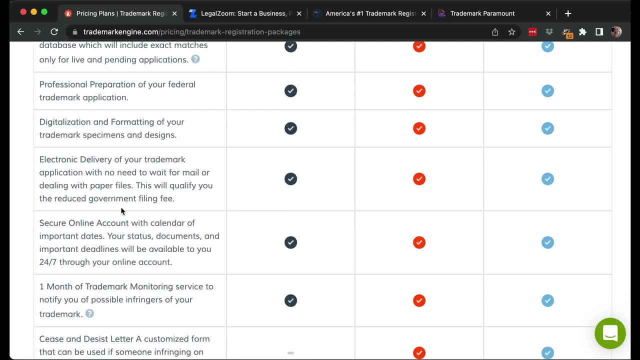 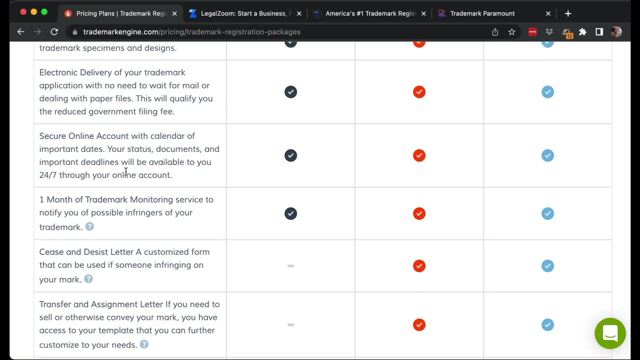 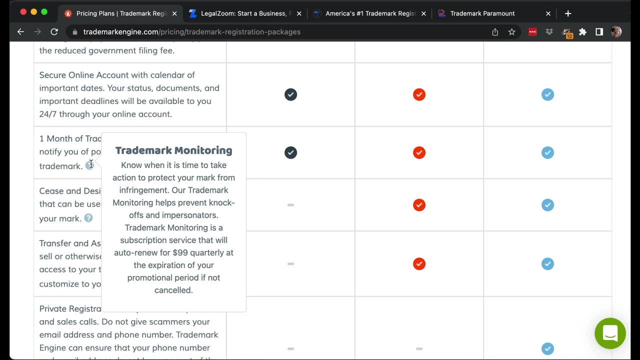 means Formatting specimens. that's just saving electronic files. that's fine. Electronic delivery of your application: Yeah, they, you should be doing that. I. you can't really file by paper anymore. You have some kind of online account, you have some monitoring that. you is a subscription service. 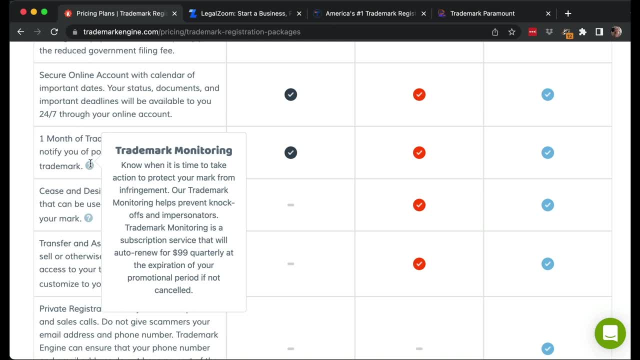 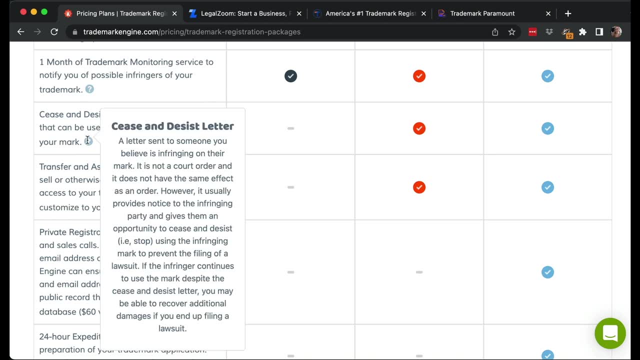 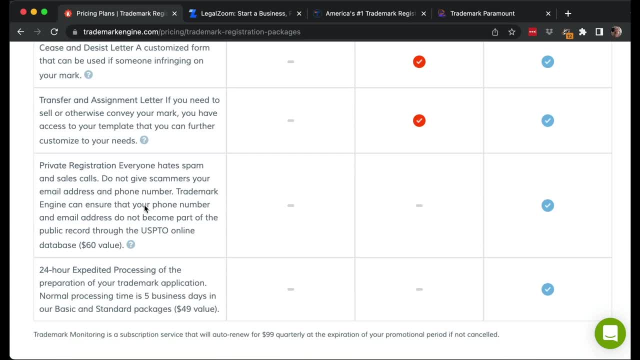 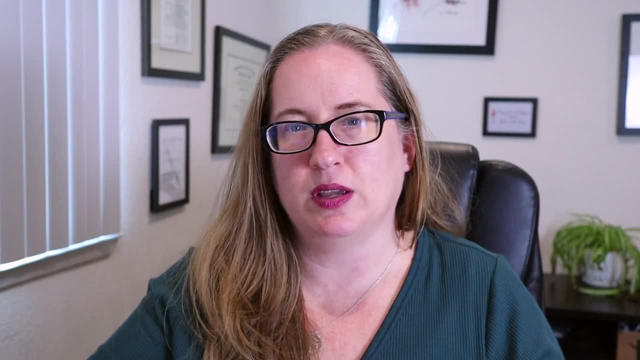 you get a cease and desist letter and they're sending you a template cease and desist letter. you get a transfer, an assignment letter if you sign up with standard. Deluxe will help you with the trademark. So if you need a trademark to transfer your trademark to another entity. 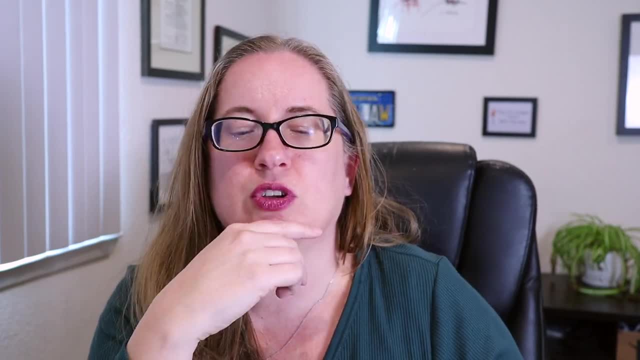 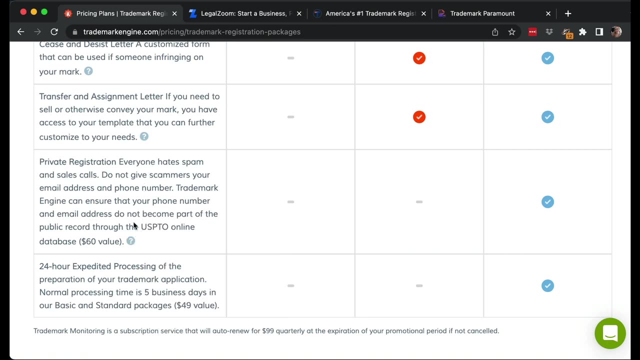 another business, you know formal LLC, whatever you have to do an assignment and private registration. So this is something that I think is concerns me. So it says: private registration is that they'll make sure your phone number and email address do not become part of the 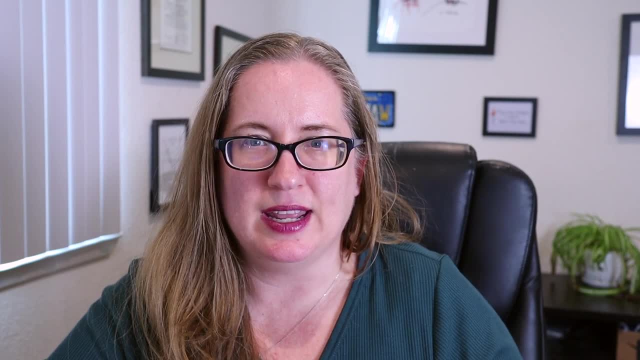 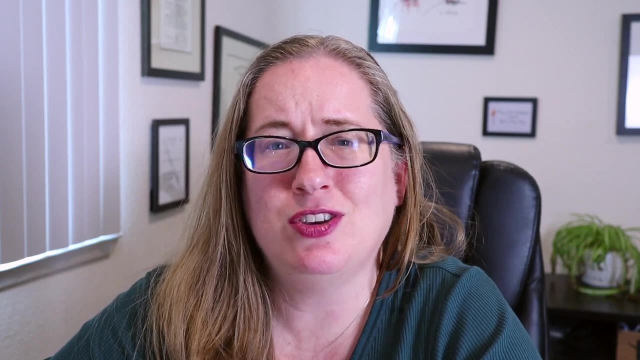 trademark. That may sound like a good idea, but I don't think it is You. if you have a business, you should have a business email and a business phone number. phone numbers are cheap and easy to get. you can get a Google voice number for nothing. A email address is very simple to get. 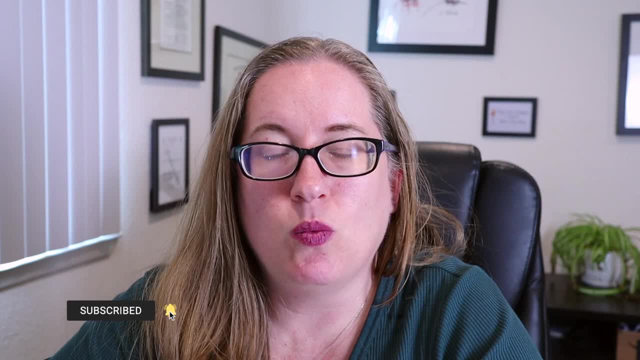 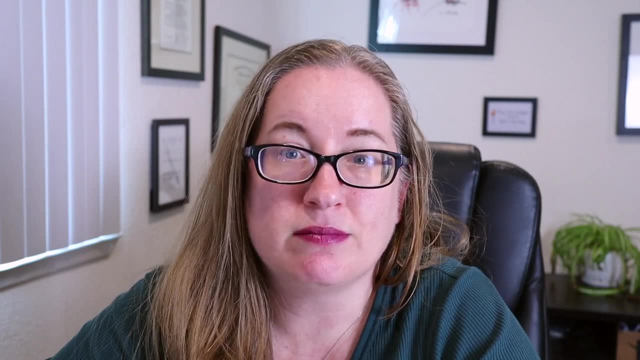 you can get a Gmail account just for this. I would never want some third party, whether they're a lawyer, whether they're a service, have the only contact information for my trademark, whether or not it's the trademark office contacting or whether or not somebody else like. 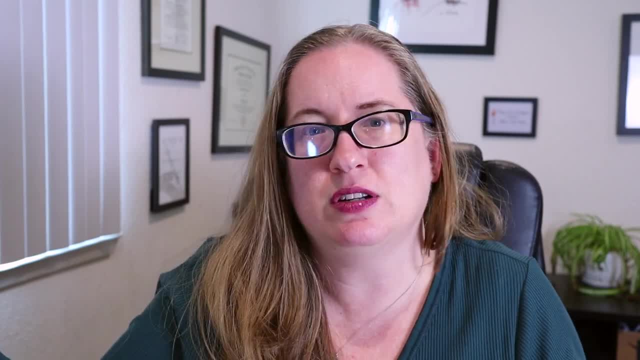 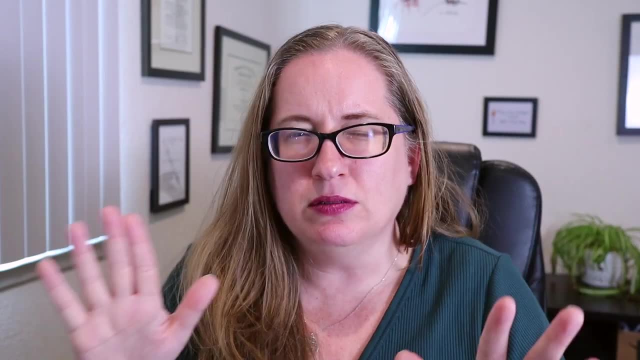 who was this company was bankrupt and then your contact information isn't on there And you don't know when the thing needs to go up for renewals or whatever. So I don't think you want this at all. It sounds good, but I think it's bad. 24 expedited hour- expedited processing- Normal processing. 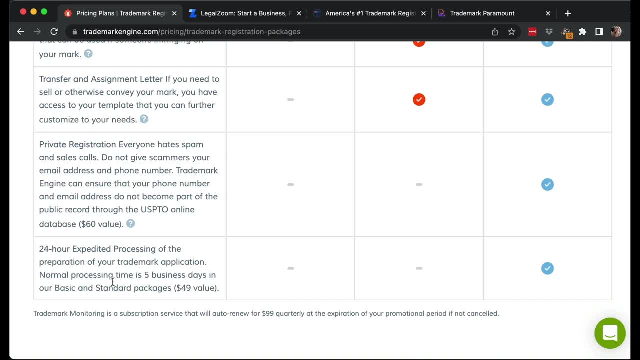 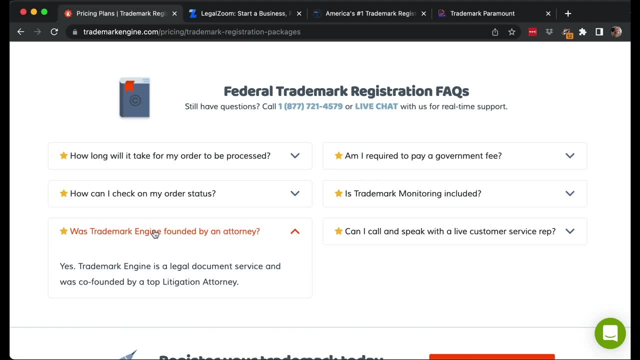 time is five business days. someone may or may not want that. That's obviously up to you. Okay, so was trademark engine founded by attorney. so is founded by a top litigation attorney, which I don't think has anything to do with trademarks. like litigation, what kind of litigation, whatever. 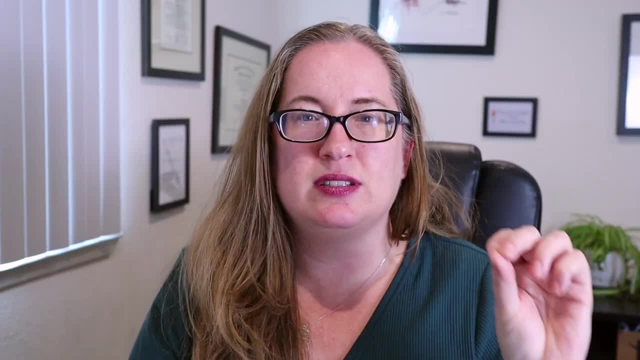 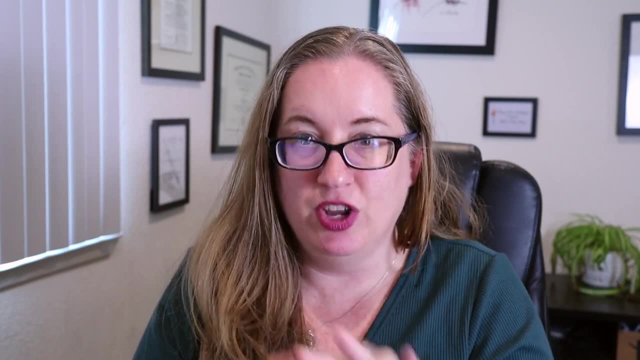 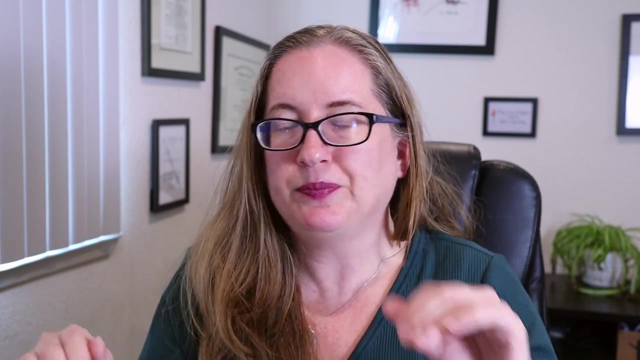 That doesn't even make me excited at all. It's a legal document service. It's not a lawyer, Not a lawyer. So they're just literally typing stuff in forms. This could be helpful to somebody where you look at the forms and you cannot deal with it. It is too complicated for you, Maybe. 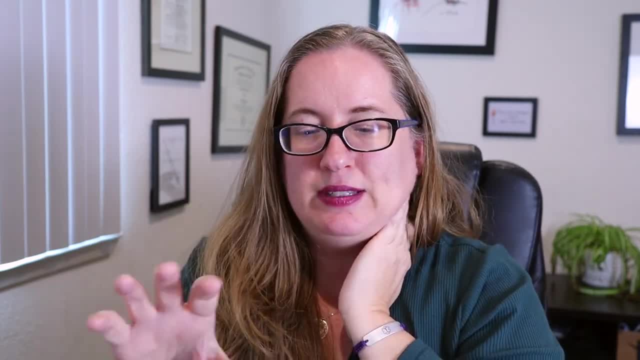 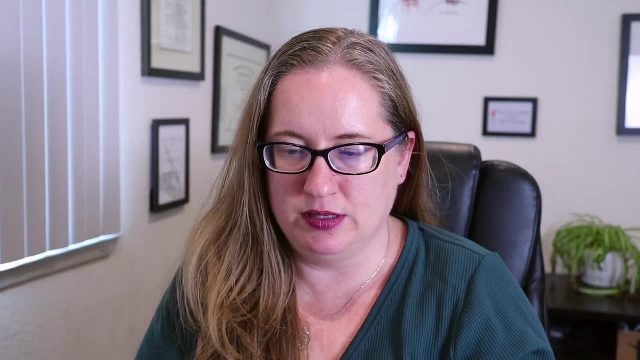 English isn't your first language. you just can't figure it out And you need someone to literally fill the stuff out for you. But you don't have the kind of budget for a lawyer, And so this is. you can get the basic package for $99 and they will handle that for you. That's obviously a very low price for trademark. work. Can you call and speak to live customer service rep? they said that they answer the phone. I haven't actually tested to see if they do. I'm not going to do that right now. You get one month of trademark monitoring. This is something that I would want you to watch out for. that they're not. 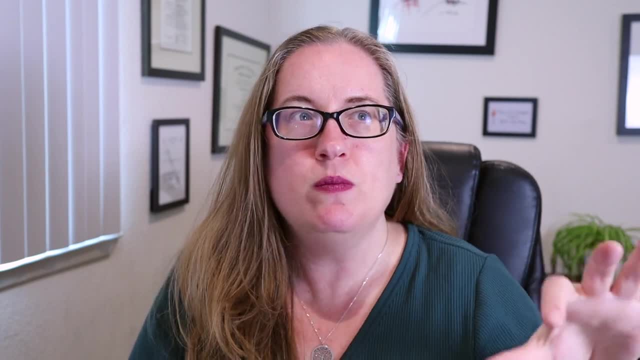 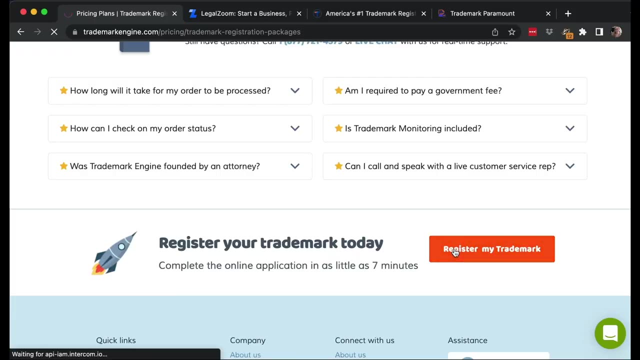 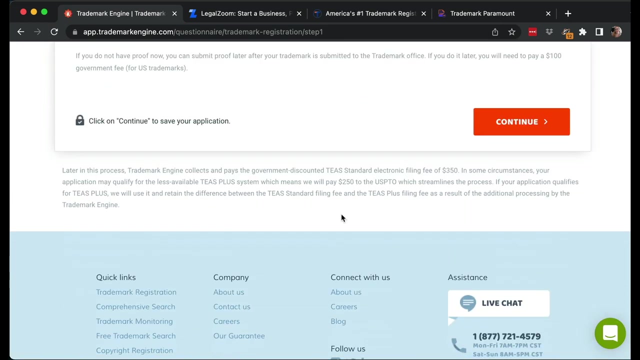 going to automatically sign you up for the $99 a quarter. You may want that, But you don't want to sign up for that accidentally, and be surprised If I click this. then what happens? I'm gonna see. Okay, then you start filling out the form for what you want your trademark to be And you're starting. to go through the process. So what happens is is that for the USPTO filing fees, trademark engine collects and pays the filing fee of $350.. Sometimes you may qualify for 250, then we will use it and retain the difference between the standard filing fee and the plus filing fee as 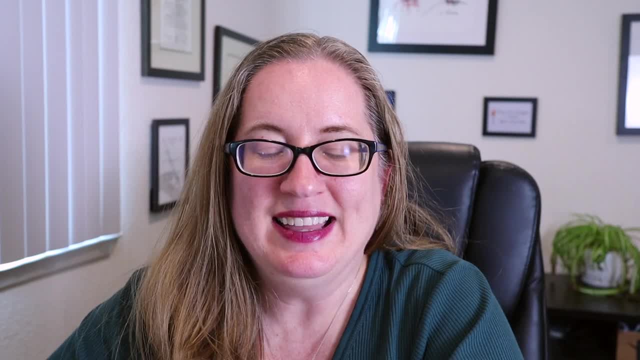 a result: Additional processing fee: The single time you'll have to file a filing fee. If you use the standard filing fee for the standard process fee, then the plus filing fee for the first three, saying what i am not happy about this. so they said that you. so here's how trademarks work. 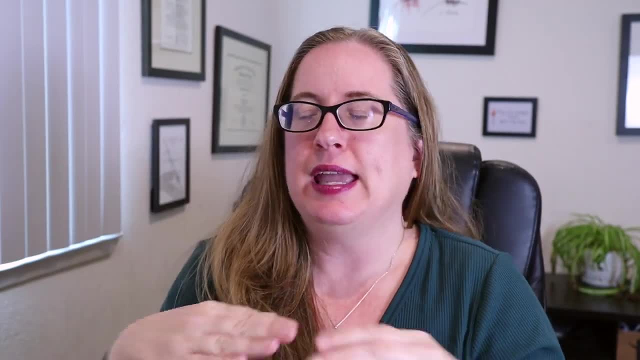 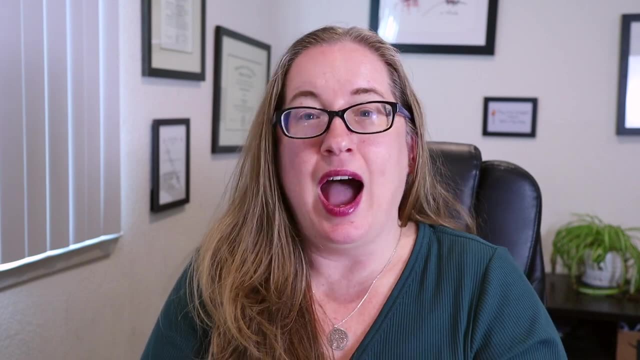 is that when you file for trademarks under current law is that there you have to write a class description, which is the description of your product or service. i recommend that people use the plus application and use it's this gigantic database of class descriptions and use one of. 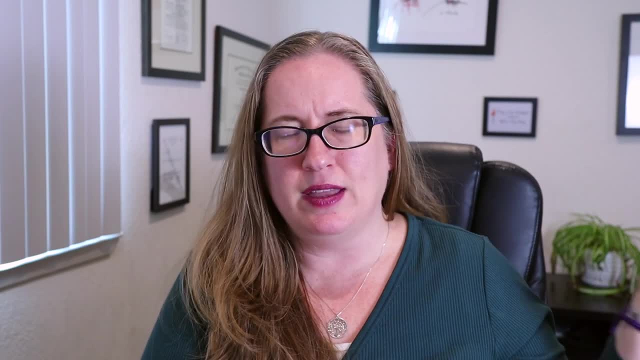 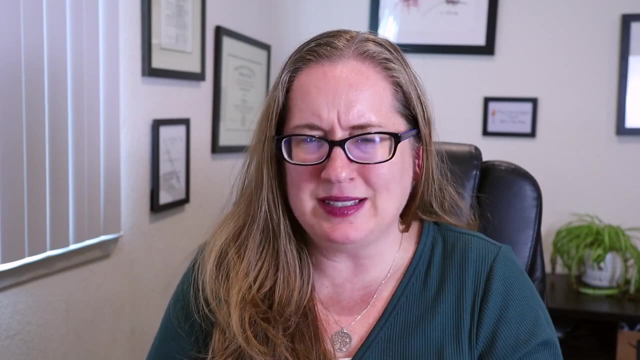 them because they've already been approved. you don't want to like write your own and then they do reject it. use one that already been approved: easier, faster and you save a hundred bucks here. they're saying that if you save a hundred bucks they get to keep it. they said it's because of 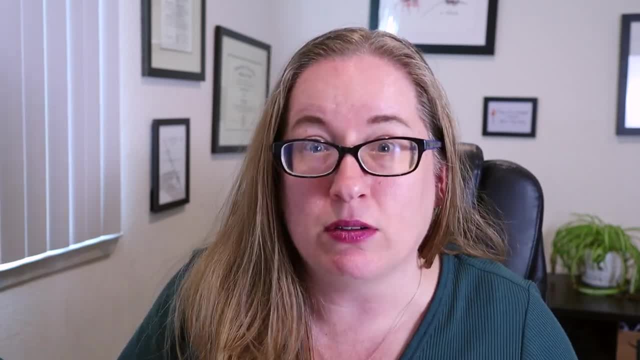 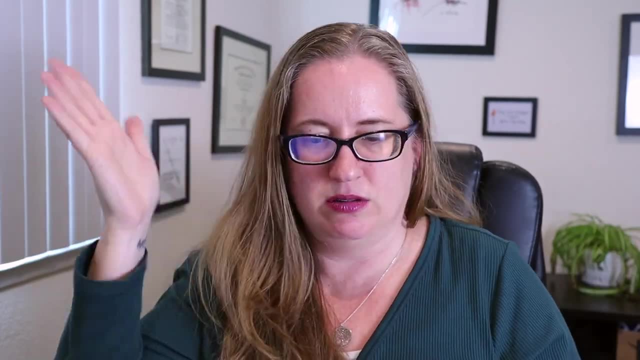 additional processing. it's not additional processing, it's less processing. so that's, that is just not good. i do not like that at all. but because they're keeping a hundred dollars of your money, i don't understand. i don't understand that. um, so i think what would happen is you go through. 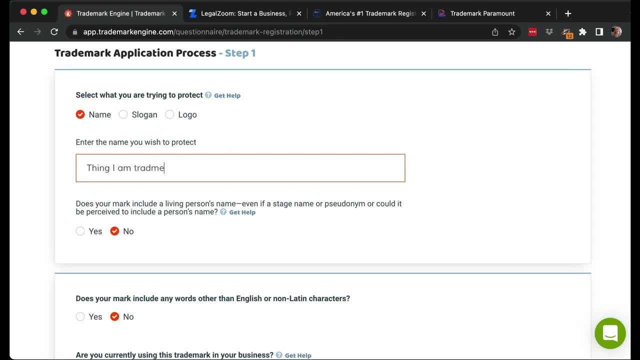 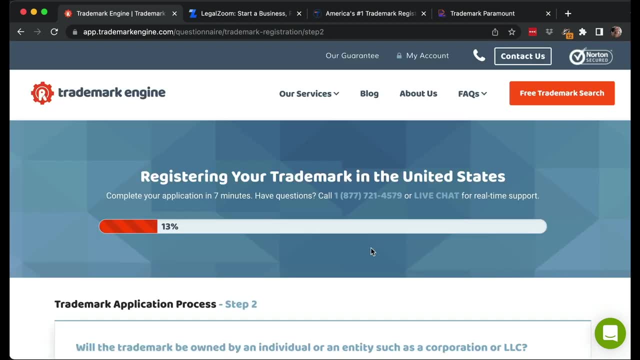 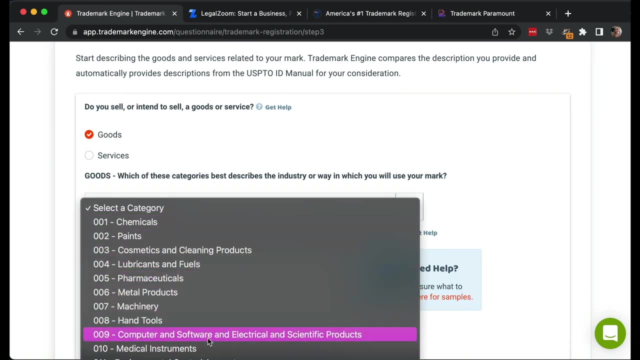 this process thing. i am trade marking. okay, this is not nothing, it's a name. we're gonna say: no, individual, individual choosing your trademark class. okay, i'm literally just gonna do. we're gonna do a podcast, whatever. i'm just fulfilling a nonsense. do we want to do? 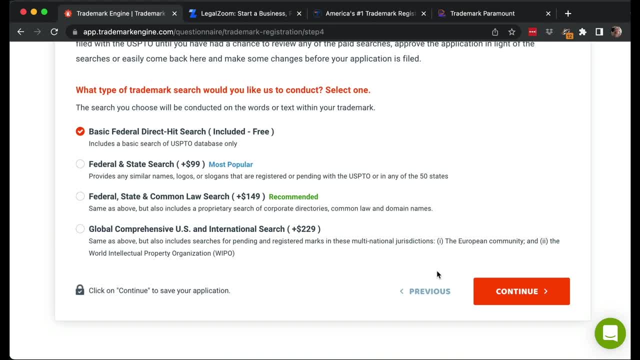 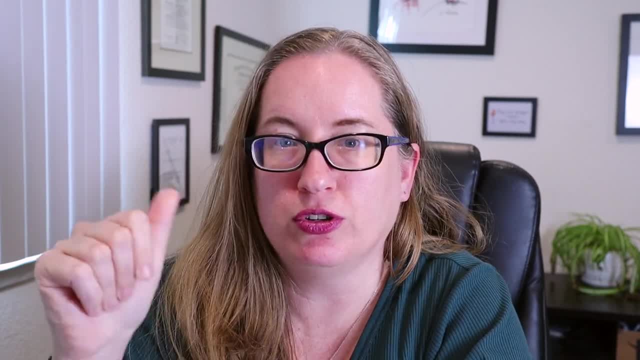 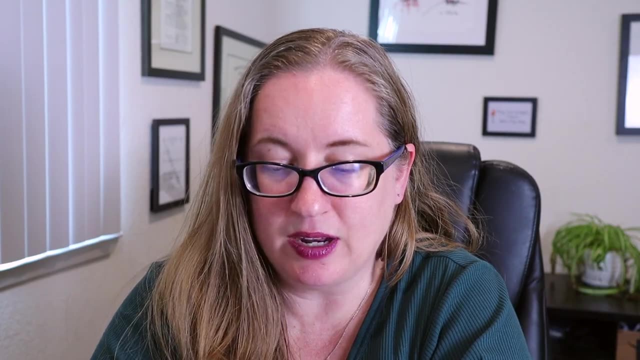 a trademark search. we're just we're not going to pay extra for this now should you do this? so here's the thing. what i recommend is that you do your own search on google and you do a search in the trademark database. so this is basic search: 50 states. i think it is helpful to do. 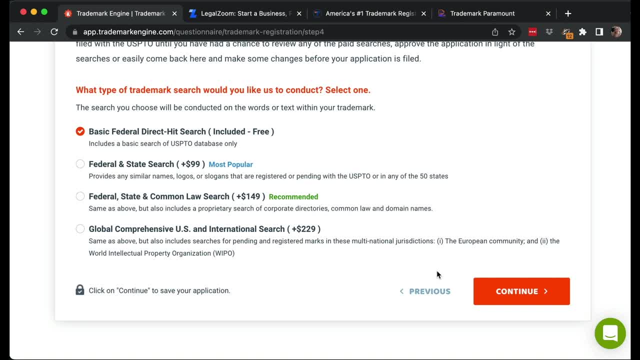 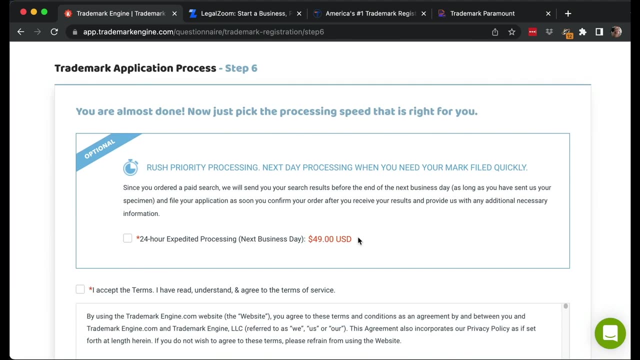 the states and common law search. if you're worried about that yourself, i think it's weird that they don't say that you're, uh, they're going to search on google, but so we're just going to do the free one. we're going to do the basic package. now pick the. if you want to do rushed processing, you need. 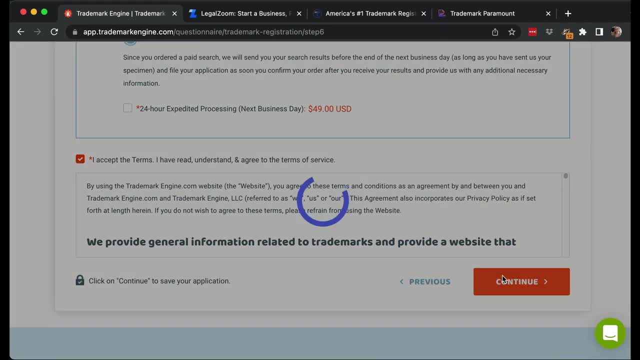 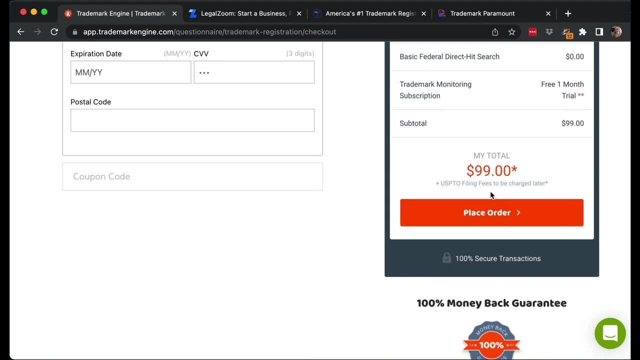 $49. i'm going to accept these terms whatever, so i'm obviously not going to pay for this. you have a trademark registration package and then it's 99 plus the filing fees to be charged later. okay, so i'm obviously not going to be doing that. right now. so i'm really unhappy about them keeping the extra hundred dollars. if you do the plus, i think you should definitely do the plus, and it seems like they don't do that and i'm not happy with it. also, the trademark engine monitoring is a subscription service that auto enrolls, so you will. 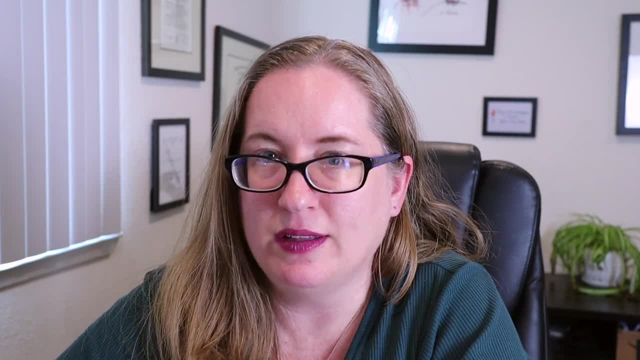 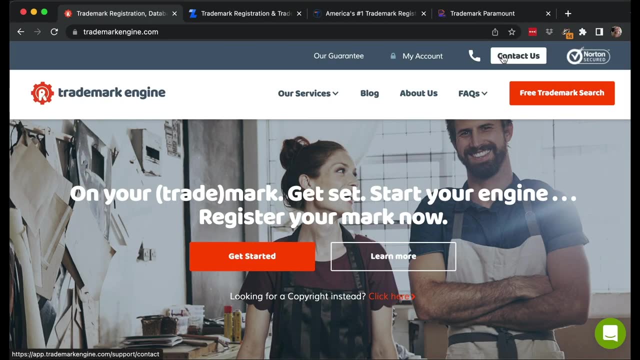 be paying 99 a quarter. you may or may not want that, but if you don't want that, you're gonna have to make sure you affirmatively cancel it. so the last thing i'm gonna do with trademark engine is do a due diligence. they have a phone here if i hit, contact us what actually happens. trademark engine. 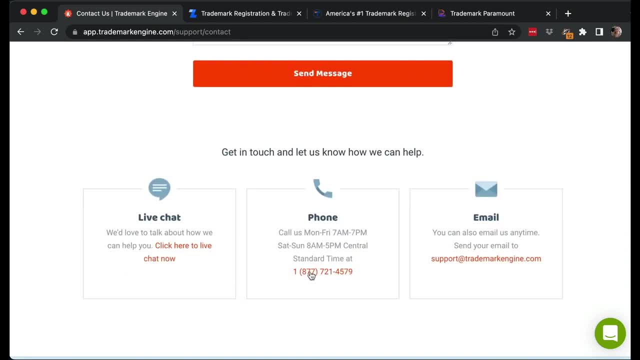 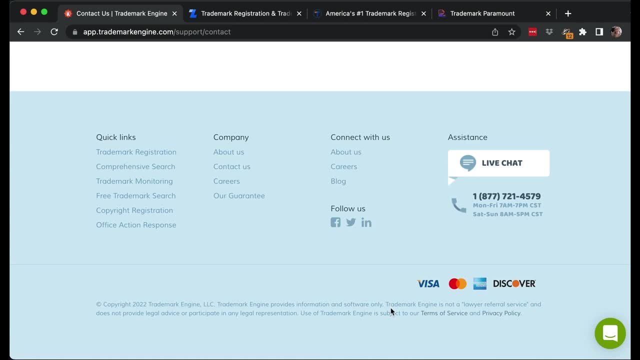 is not a law firm. it's not legal advice. all right, they have a phone number. it's an 877 phone number. that's a free phone number. i think they have an email. they have a live chat. let's look, i'm going to try to figure out who are these people. company about us, so you click on about us. 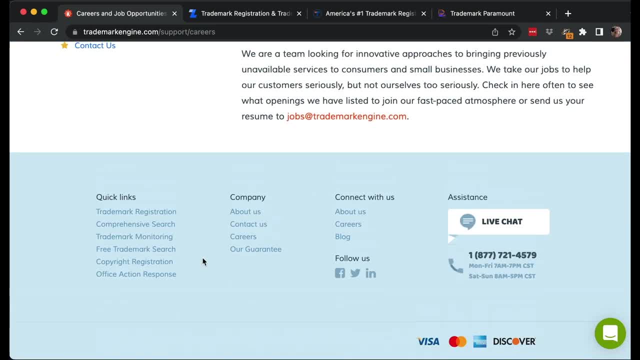 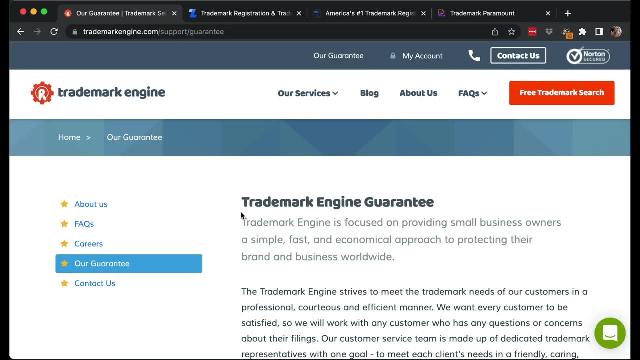 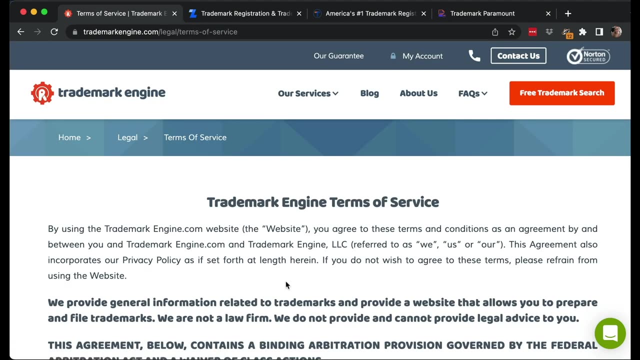 just has some generic stuff. careers: you can send them a thing about their jobs. contact us. we already know this is just a form. so our guarantee: what kind of a guarantee do they have if you don't think that they did a good job? they have a guarantee. i say nothing about where their business. 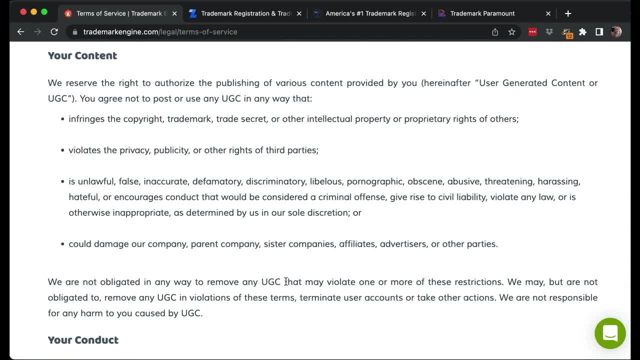 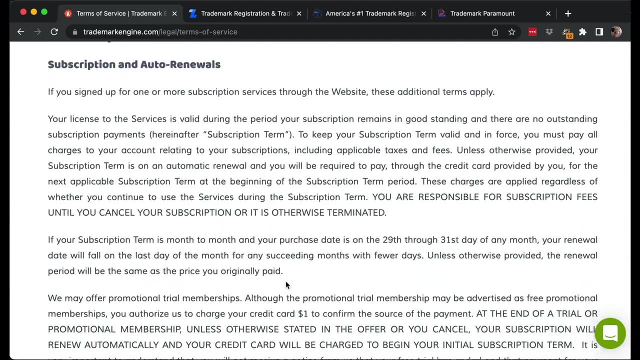 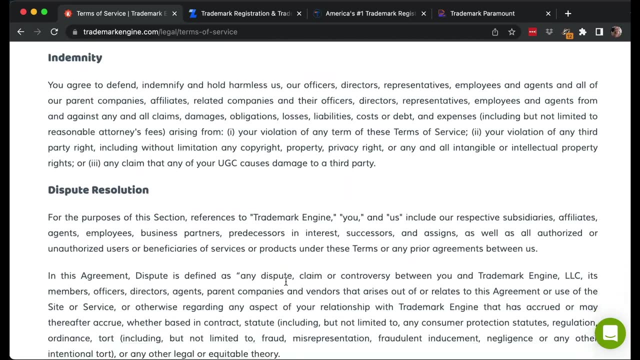 is okay. so here's a terms of service, and now what i'm trying to find is: who are these people like? where are they located? what countries are they in? what state are they in? uh, all this stuff, they have no rules, blah, blah blah. they do logo designs, which is interesting and strange. um, okay, if you're. 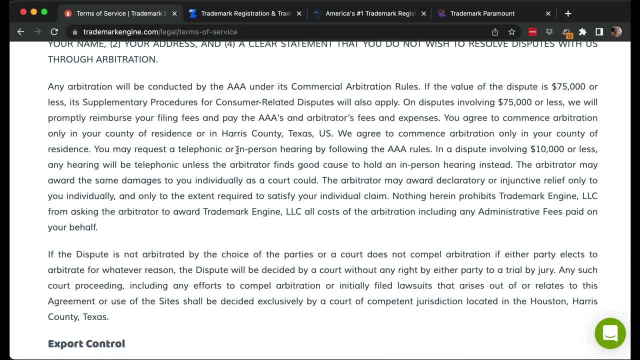 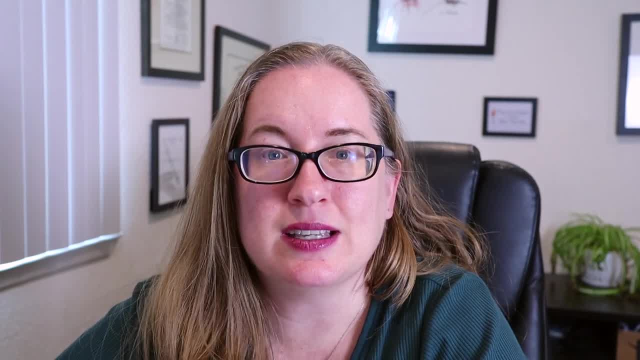 opting into arbitration. okay, so here to agree to commence arbitration in your county of residence, or harris county, texas. that means somebody's in texas, so they're probably here in the united states- at least somebody's in the united states- because they want to do any legal dispute. you. 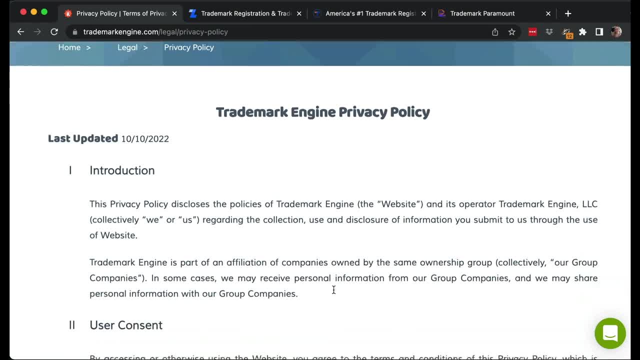 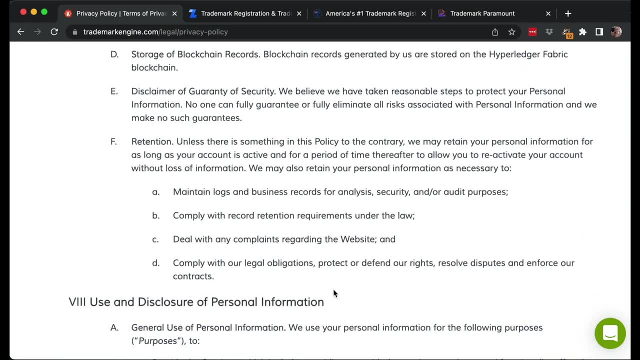 have with them is going to be in texas and their privacy policy. i don't see anything different. i mean, i'm glad they have a privacy policy, but i don't know what else is blockchain stuff? i mean, what does that have to do with anything? so, by the way, they can share your 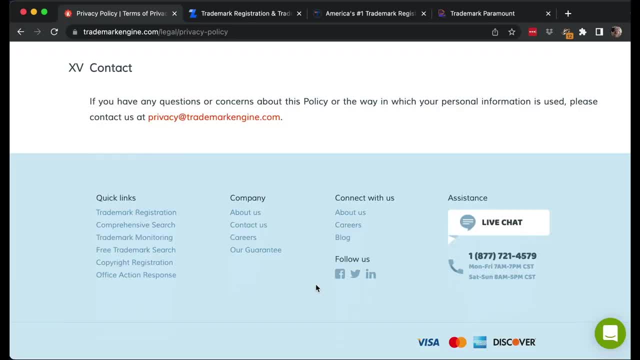 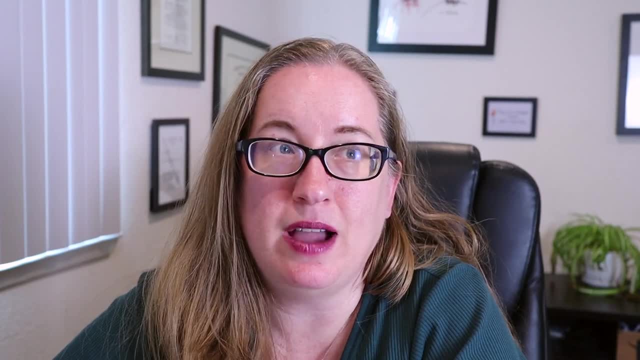 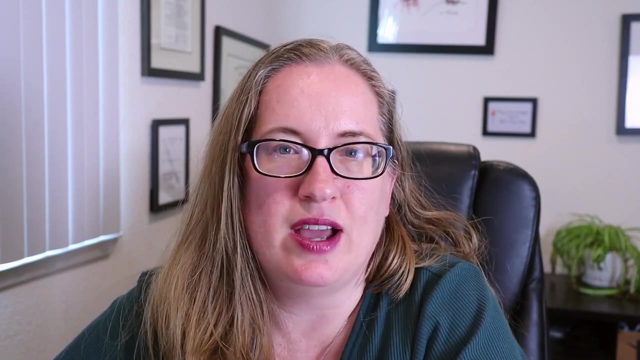 information with group companies, with business affiliates. they don't have any kind of address. they don't have any kind of information about where they're located, except the fact that their choice of of jurisdiction is in texas. but there's no reason to not have an address on your website. 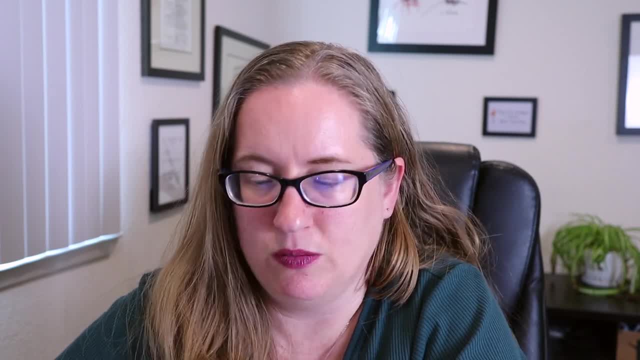 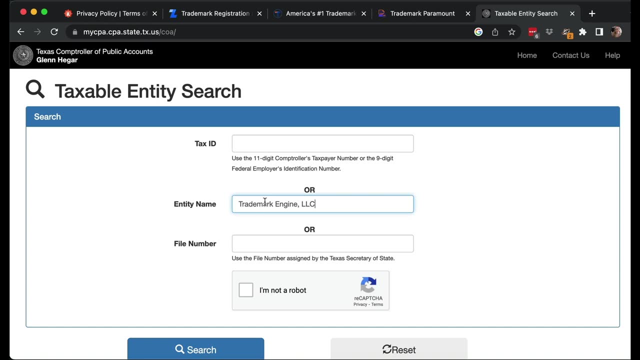 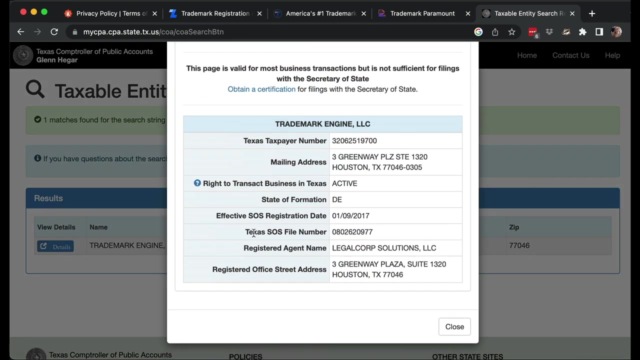 it's a virtual mailbox address, i mean it's. i think it actually is slightly weird. we also don't know what state the llc was formed in. i'm assuming it's in texas. i would look up entity name, let's see if we can find this. so, trademark engine llc. aha, i don't have an address. they were formed in delaware. 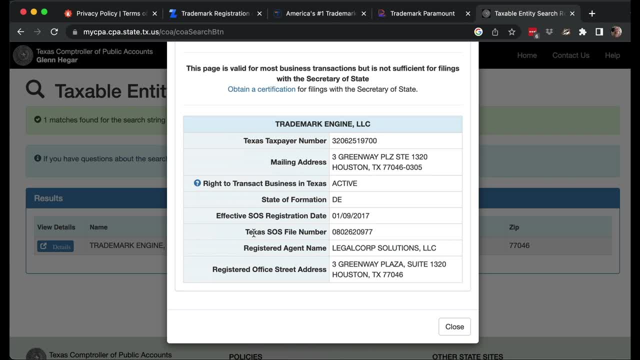 and then there's their address in houston, texas, and the registered agent name is legal corp solutions, which is not them, which is kind of interesting. um, so this is where they're actually located, and then here i can be really sneaky. i can actually look that up. 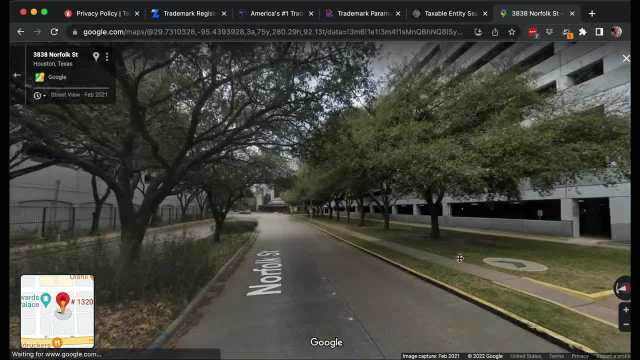 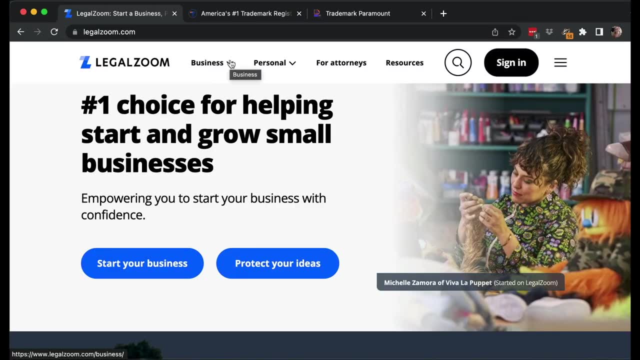 let's see what that is: some sort of corporate buildings. so there's a good chance that are actually in there. that's good. let's move on to legal zoom. now. legal zoom: i actually i have never used them to file trademark application, but i have used them to do a. 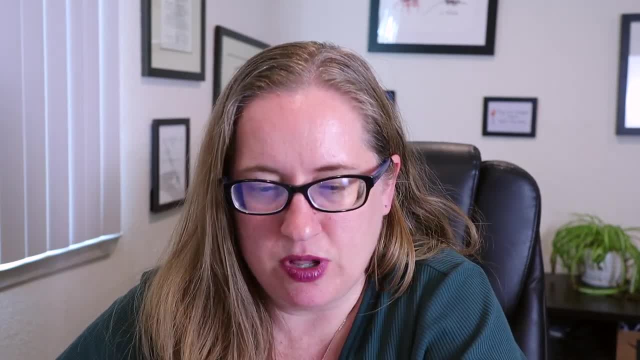 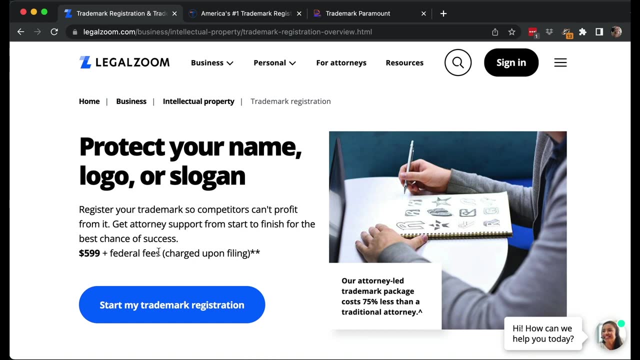 trademark search before. so i'm familiar with how they work. so first we'll click on business, first trademark registration. okay, so here 599 plus the federal fees. okay, plus federal fees. totally makes sense. it has two stars. two stars always makes me nervous. what does the two stars mean? 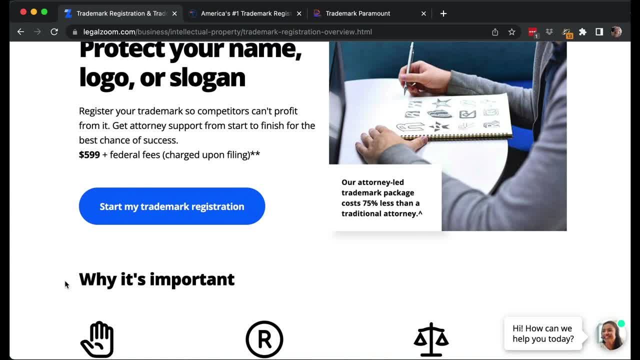 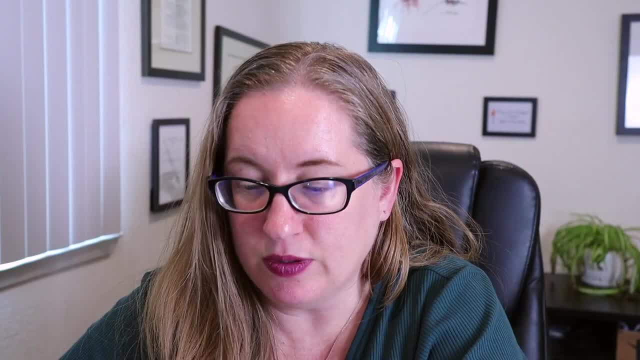 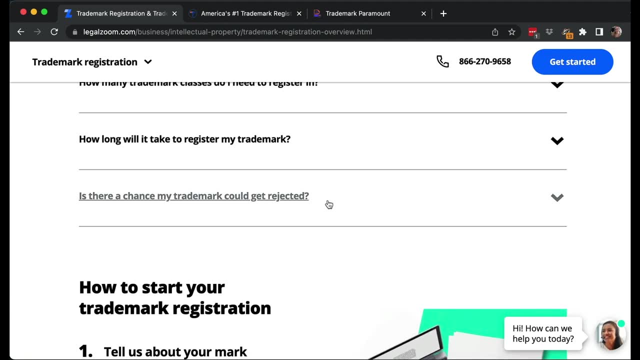 let's find where the two stars are defined. no idea, i don't know whether two stars are fine. oh, okay, it says this is a attorney-led trademark package. i don't know what that means. we're going to try to find out. uh, why do you want a trademark? is there a chance that we'll get rejected? 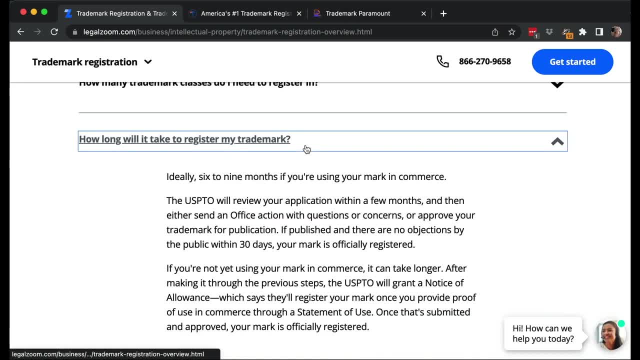 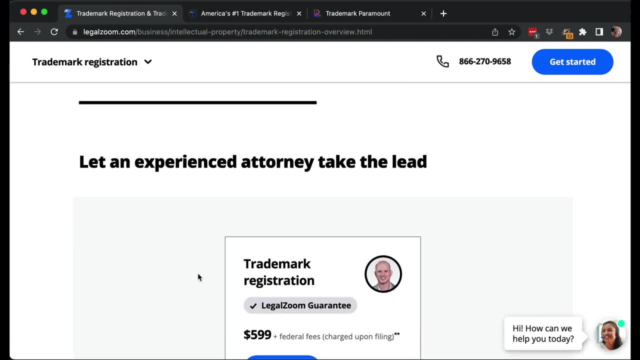 yes, how long the register? six to nine months. it will take way longer than that. that's just because they haven't updated their things. so it says: let an experienced tourney take the lead. all right, so for legal zoom their trademark registration: 599 plus federal fees. attorney. 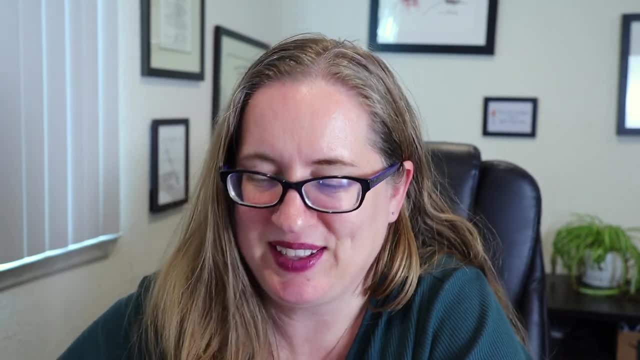 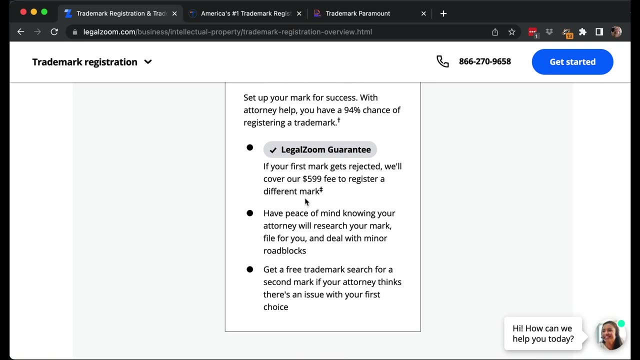 help. you have 94 chance of registering a trademark. we can talk about that later. um, if it get your first market's rejected, we'll cover our 599 fee to register a different mark. that's actually kind of an interesting. reason why something is rejected is that you can do a lot of. 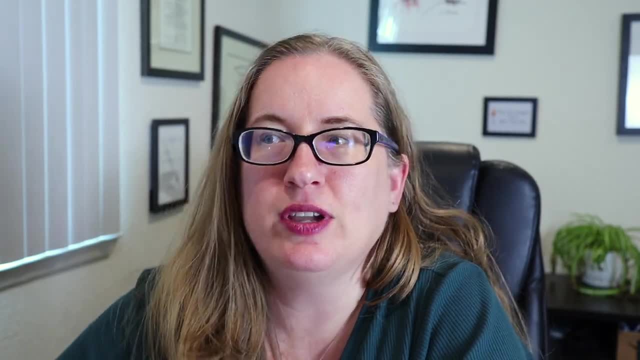 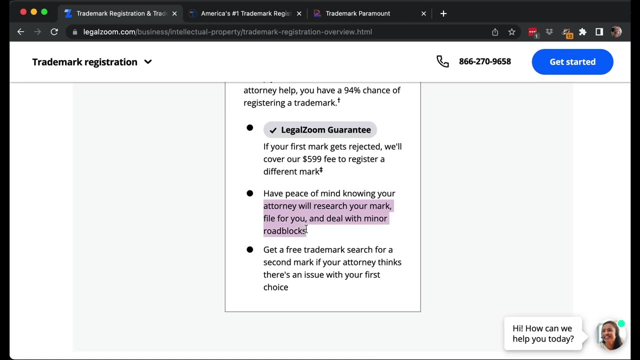 way to do a guarantee is that you don't get your money back, but you get a credit for the next trademark, um. an attorney will research your mark file for you and deal with minor roadblocks, get a free trademark. search for a second mark if your attorney thinks is an issue with your. 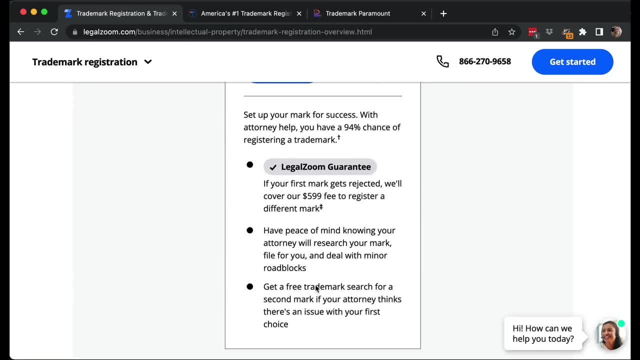 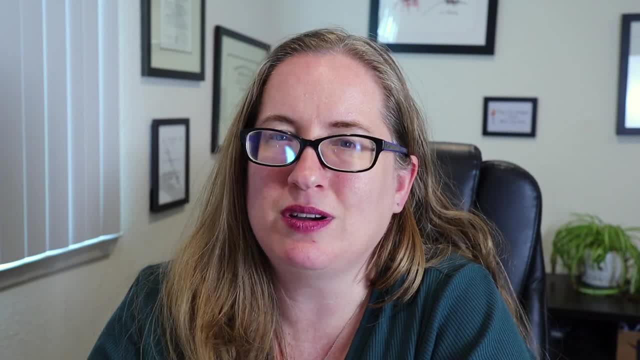 first one. okay, uh, because that actually is one of the things that's an issue is, sometimes you'll hire someone to file trademark application for you, but you really want a consultation before they go ahead and file it, because maybe it won't work. all right, they say they've done 320 000. 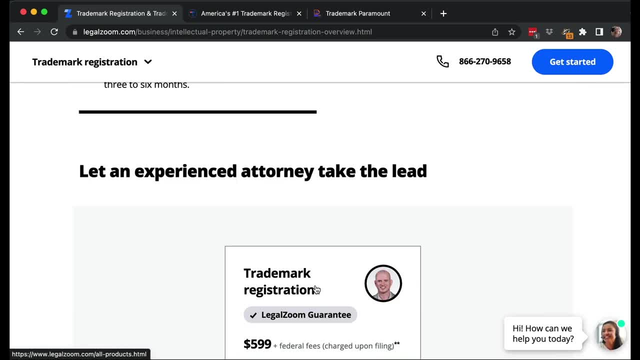 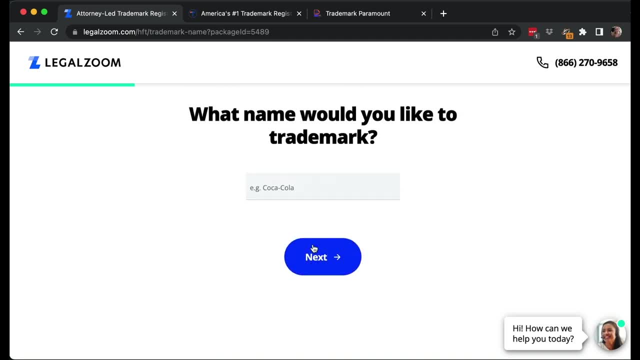 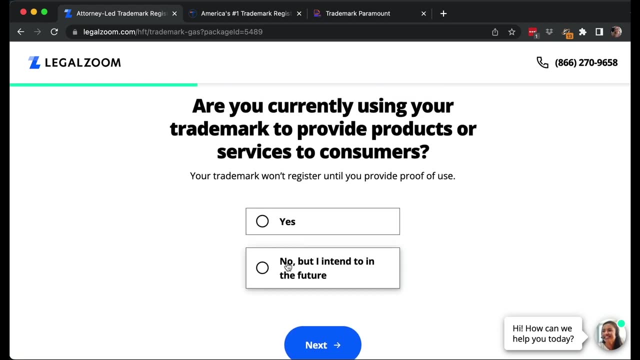 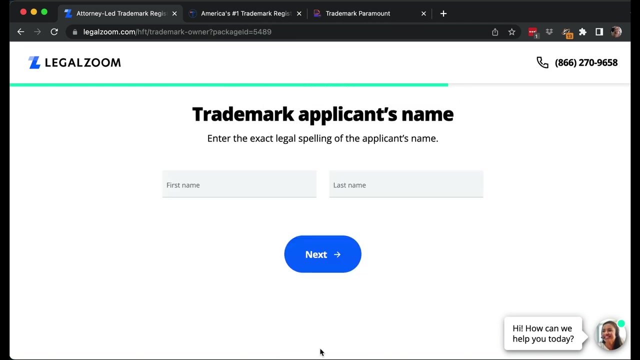 trademark applications. okay, agents are based in the us. all right, start my trademark registration. all right, we're going to start. now see what happens. business name or product, product thing to trademark- it's a terrible name, um are you currently using. we're going to say no description of goods podcast, who owns the trademark? we're just going to say me. 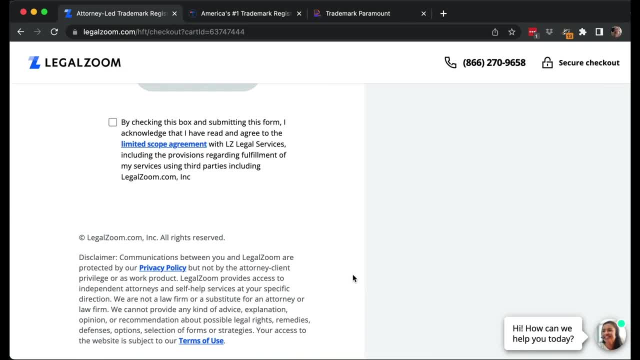 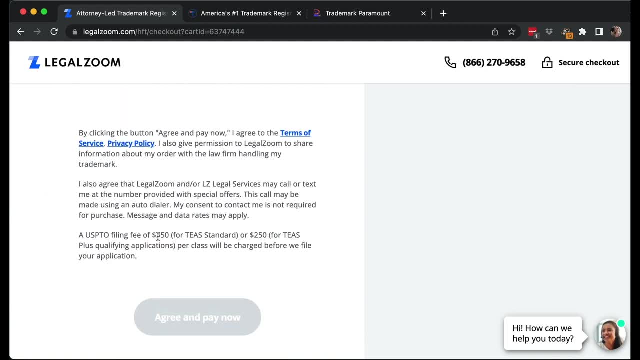 all right, assembling the package. okay, i'm obviously not putting that in there. let me go see what the terms of service and stuff are. okay, usp, uspto filing fee of 350 or 250 will be charged. before we file we can call and text us. look at the terms of service and the privacy. 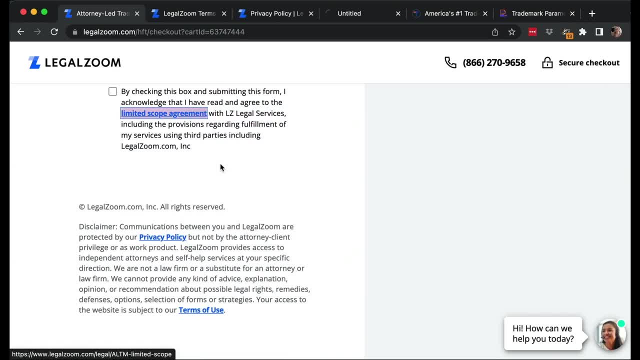 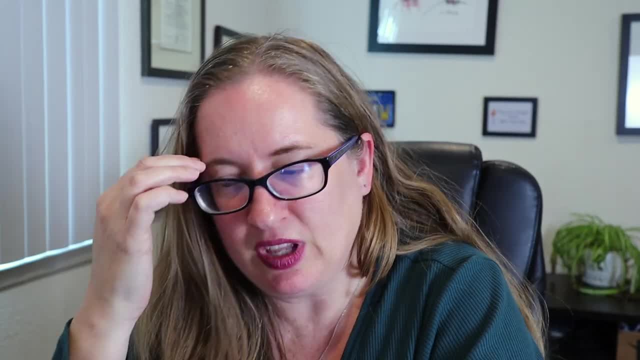 policy in a sec, i'm agreed to a limited scope agreement with something called lz legal services, i'm assuming. ah, so lz legal services is there are their lawyers. now a limited service agreement. that isn't inherently a bad thing or anything, is that when you're hiring a lawyer to do something? 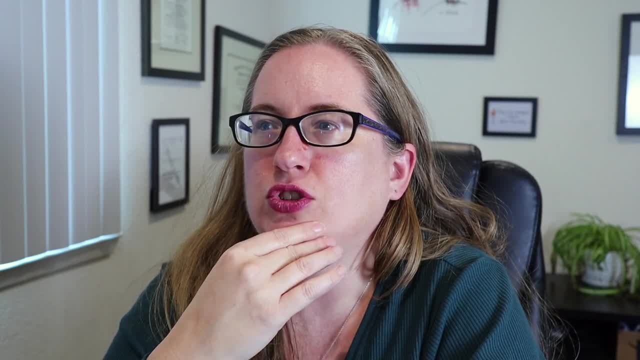 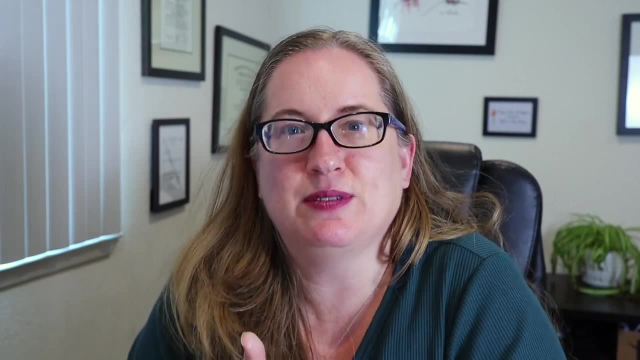 really, really small for you. like, let's say, uh, back when i used to do quick calls and and someone was just doing a 15-minute call with me- i'm not like representing them in everything you know, i'm just giving them 15 minutes of advice. so it's a limited scope agreement. so if you sign up for this, you are. 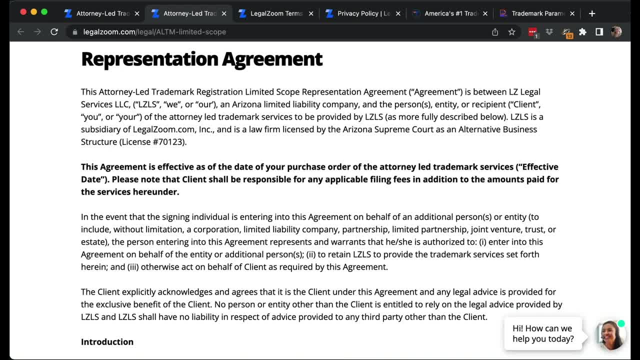 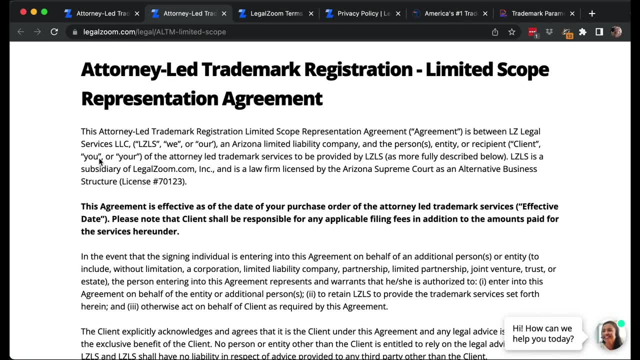 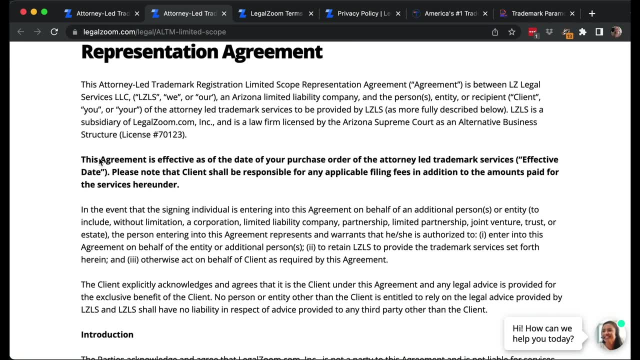 actually purchasing attorney-led trademark services, which is a very interesting like way to phrase. it is not legal zoom, it is this. what is it? lz legal services, an arizona limited liability company that is, you're having a limited scope representation with um. there's attorneys own equity in legal zoom. blah, blah, blah. 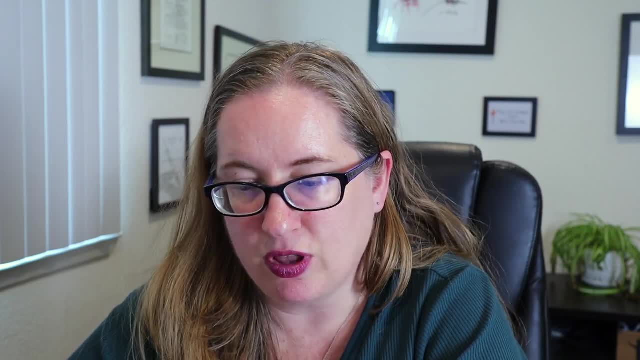 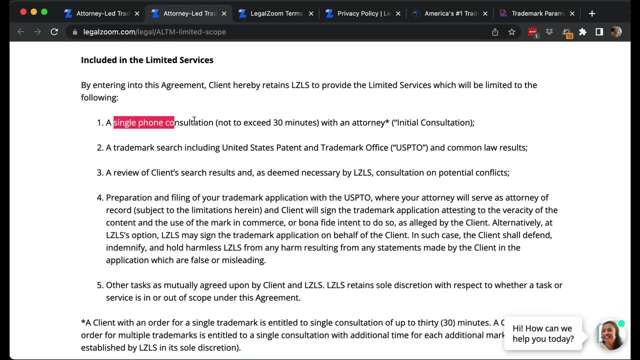 they're not representing you generally in trademark matters or intellectual property matters, but only very, very specific things that you sign up for, which makes sense. so here's what you get: you get a single phone consultation, not to exceed 30 minutes. you get a trademark search, including. you're going to get 30 minutes and also you're going to get an annual consultation. 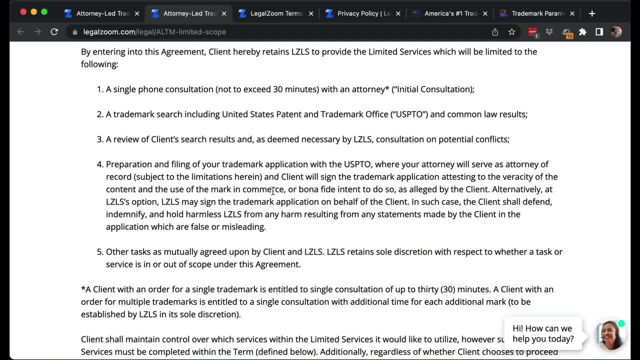 USPTO and common law results, a review of it and, as deemed necessary, consultation on potential conflicts. preparation and filing of your trademark application, where an attorney will serve as attorney of record. So this is very important for someone who is located outside. 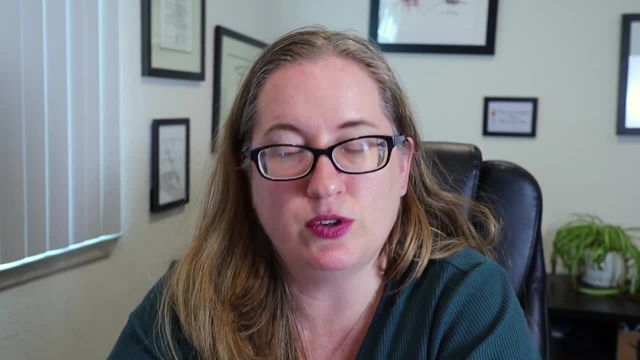 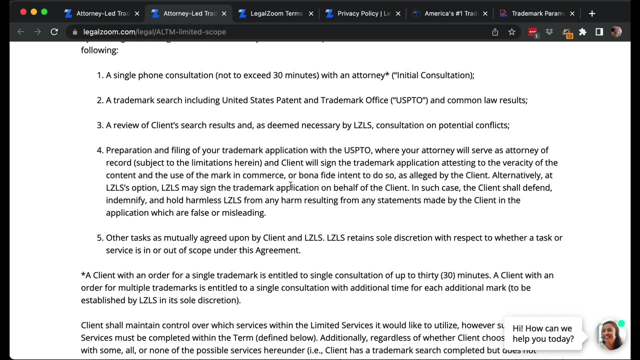 the United States. They're going to be your attorney of record, So this will work for those of you who are located outside the United States, And either the client can sign the trademark application or the attorney may sign the trademark application. I think it may depend on the. 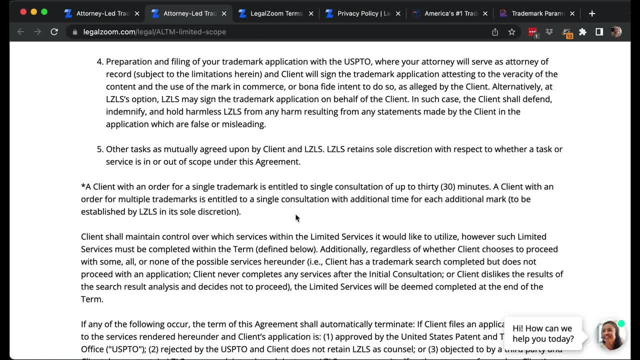 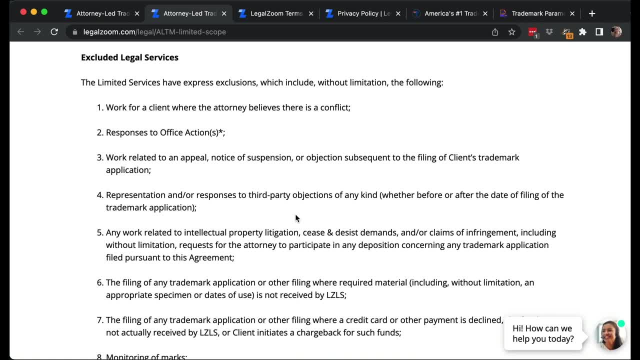 situation. If you sign up for multiple trademarks in your package, then you get additional time, which makes sense. Anything else- responses to an office action, other work etc- is not included here. So- and this is something that is going to be true most like with everybody, I actually don't. 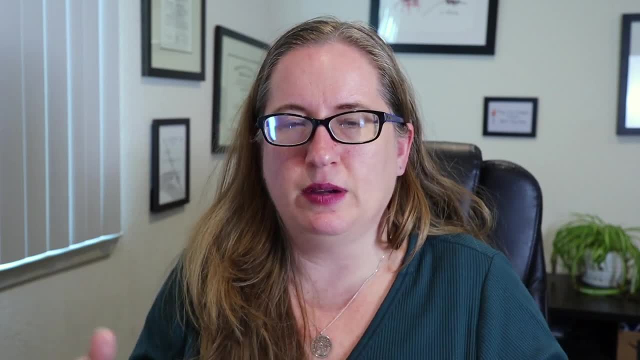 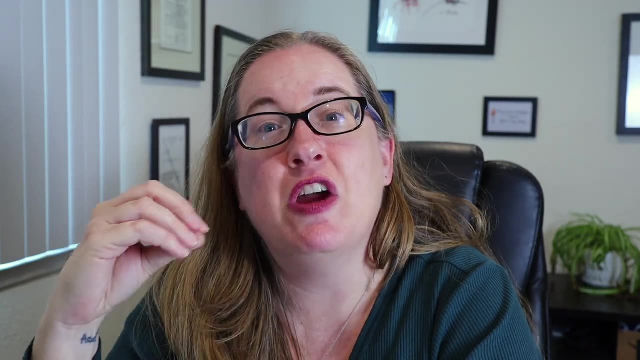 know yet, but this is something that makes sense- is that you're just signing up for them to file your trademark, not to respond to an office action. I think one of the things is, some office actions that come back are very, very, very, very simple to respond to. 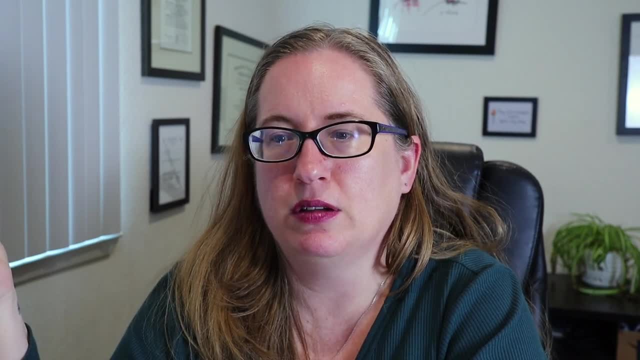 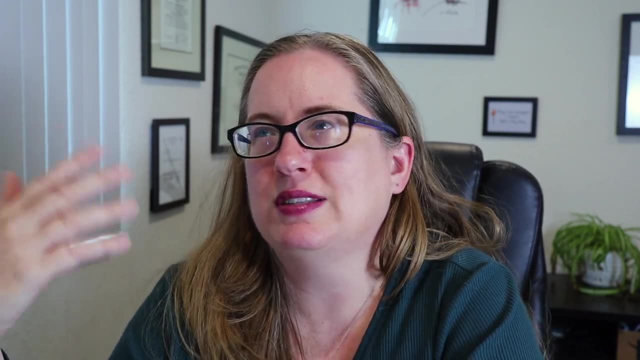 It's like that you need to make some kind of like: just change how the commas are in your description, You need to use a little bit different of a word, You need to send them a file because the file was corrupted- like just really simple things to do and charging extra for that Having. 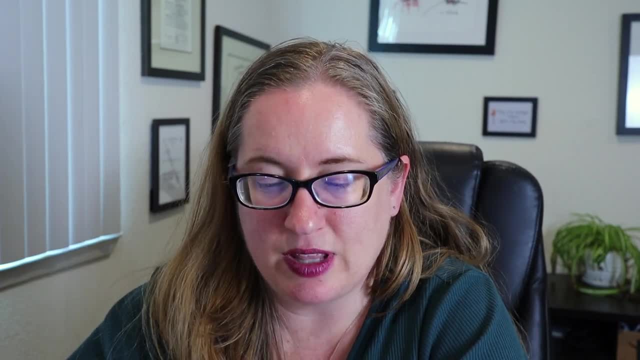 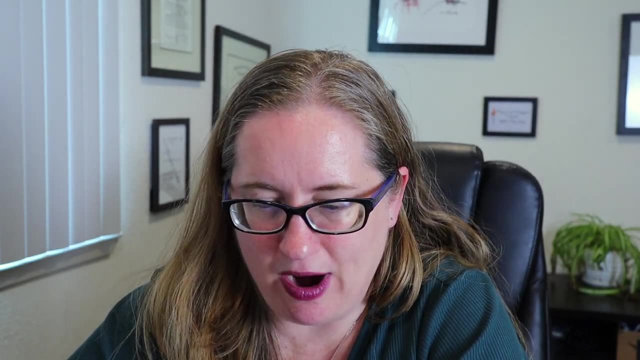 that not be included. you know it's. it's a way decision that they made something to be aware of. I don't know exactly what happens. I don't see them saying you know what their hourly rate is for the other things they charge. 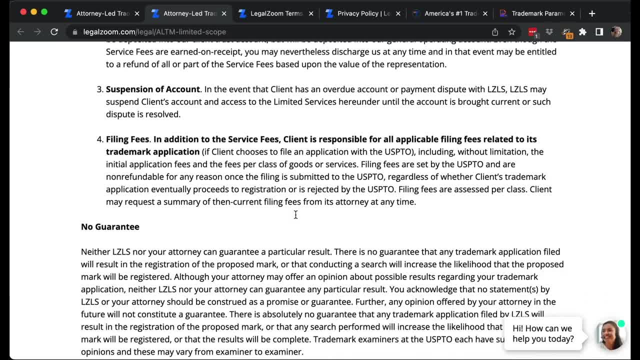 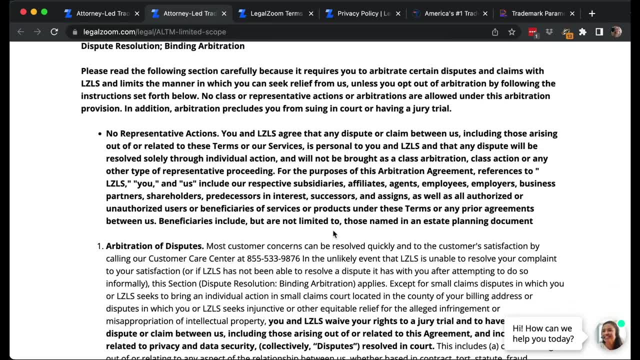 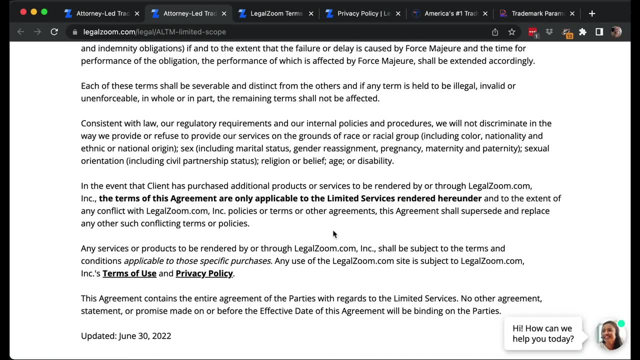 Um, I don't see any fees. um, in your client responsible for filing fees. they're set by the USPTO. There's no guarantee dispute resolution of that. That's normal thing to do. I don't see them saying what their fees are in this agreement Like. what I mean is what their hourly rate is, If you need. 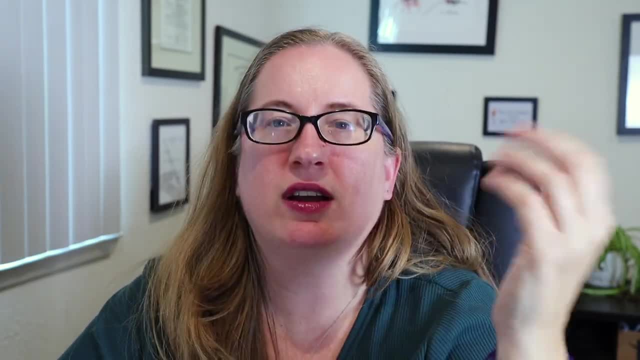 more work. I'm not sure what that is. So LegalZoom. LegalZoom is a giant company. I'm not doing a huge amount of due diligence here on them because I already know them. They're a legitimate company that actually you know they're a legitimate company that actually you know they're a legitimate. 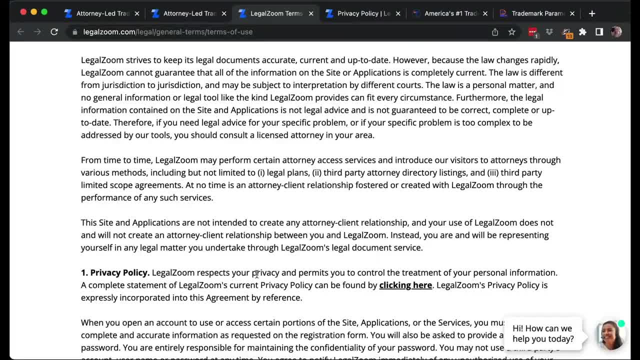 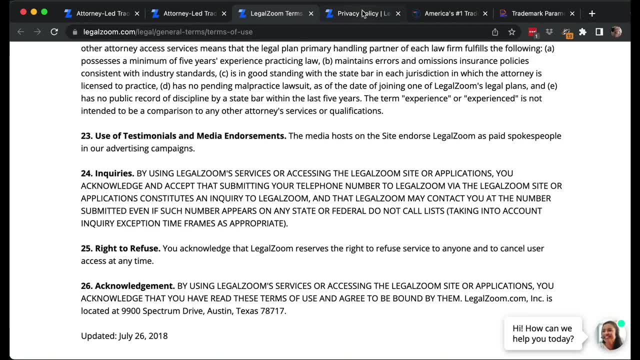 company that actually exists, Um, and they have offices and everything. Here's their big giant terms of service. You can go all the way through it. Um, you actually have their address at the bottom of it. They're in Texas. Um, they have their privacy policy. One thing to be aware of. 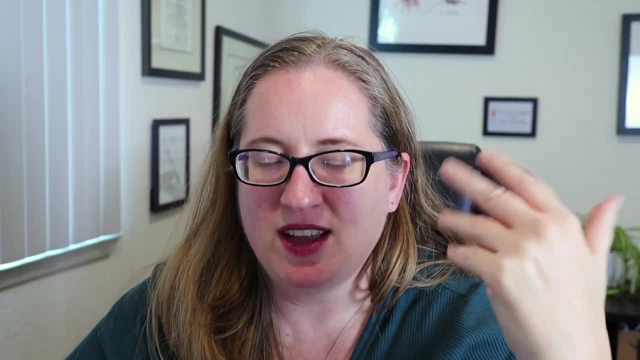 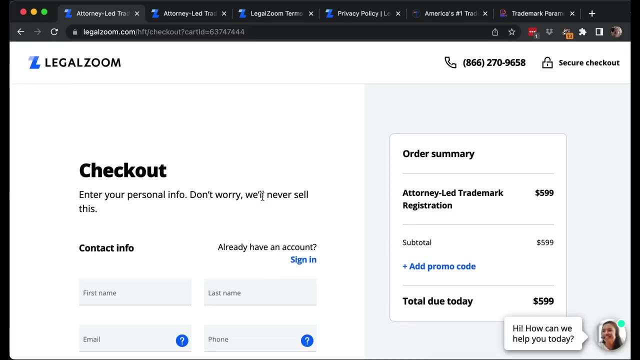 is, if you do buy something from LegalZoom, they're going to try to sell you all kinds of other things, but uh, just something to be aware of, Okay. So I'm obviously not going to pay for this, but that's the basic thing for LegalZoom: $599, which is fairly reasonable to actually 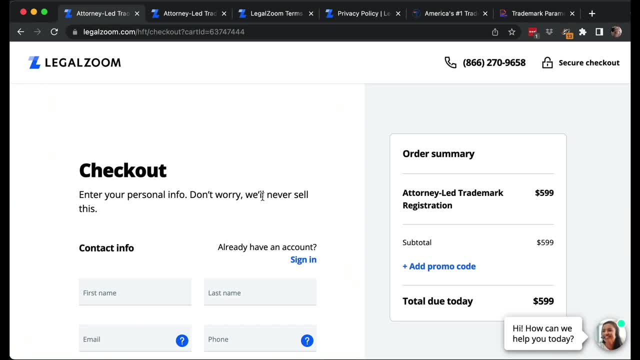 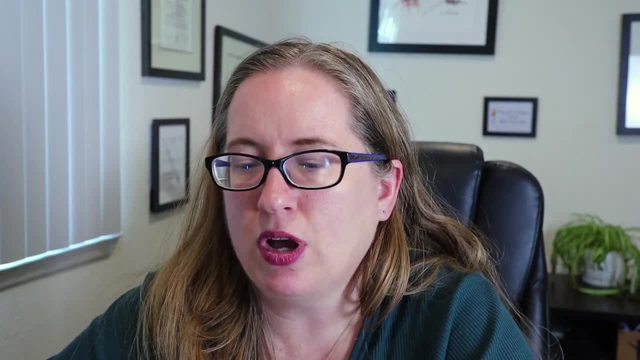 get 30 minutes call with a lawyer, and a lawyer is going to be on record, So this would work for you if you're outside the United States. So next we're going to look at Trademarkia. I was originally aware of Trademarkia a few years ago as a place to do searches for trademarks. One of the nice. 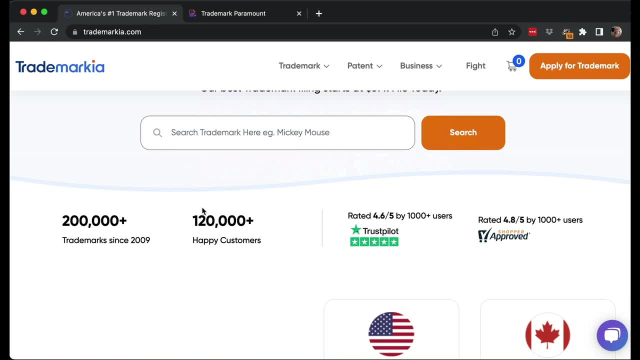 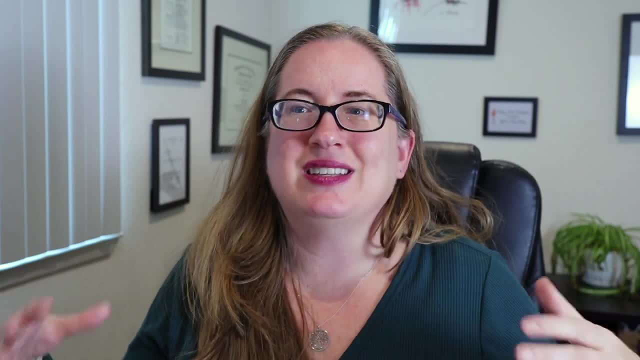 things that you can do searches on here for free that are searching in other countries. So sometimes if I need to do a trademark search in like a whole bunch of different countries, I'll come here and do a bunch of my trademark searches because it's easier than signing on to the trademark databases. 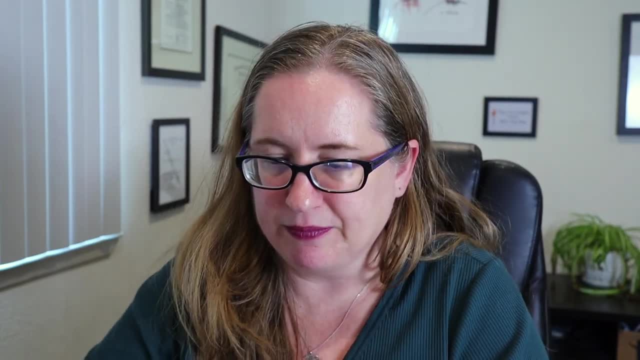 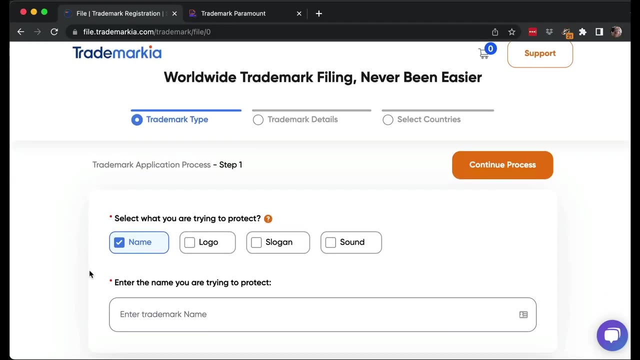 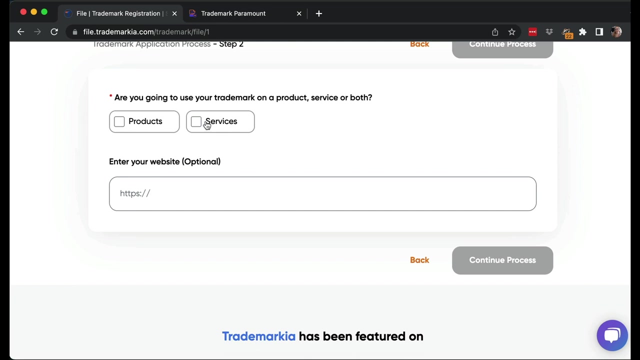 of many, many different countries And they have a search engine that's just free. but let's look at actually hire them to do a trademark registration. So click on trademark registration. So let's just say thing to trademark: Um, have they actually said how much it's going to cost? Um, we're going. 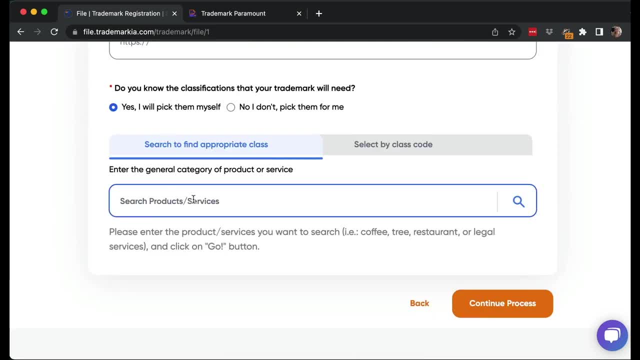 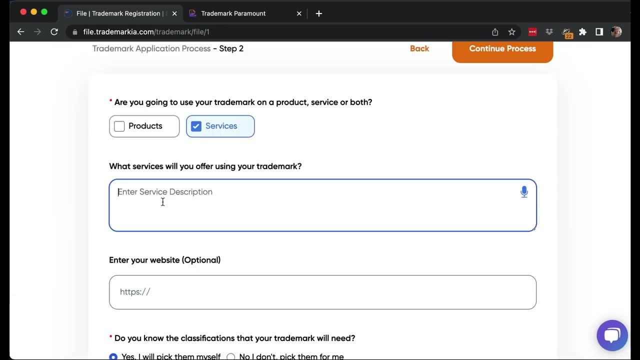 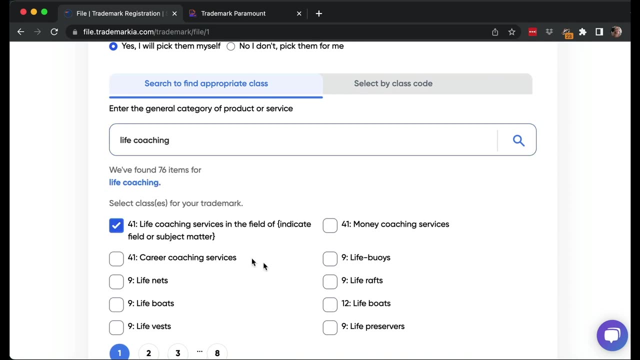 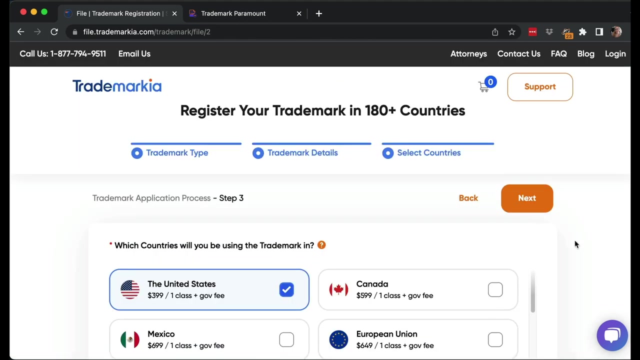 to do it for a product, um, a podcast. That's just weird. Life coaching, Let's do that one. This is actually kind of confusing because I I think a lot of people aren't going to really know what to put here. Okay, All right, So how? what is the fee? The? 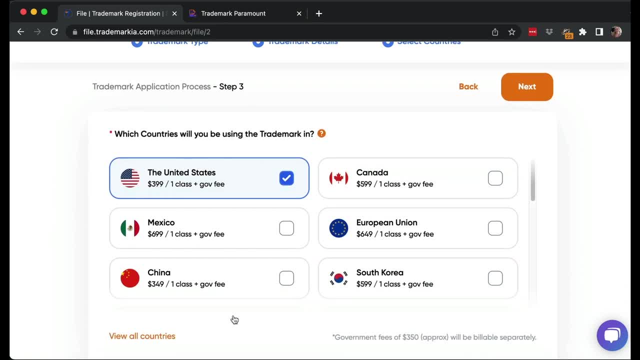 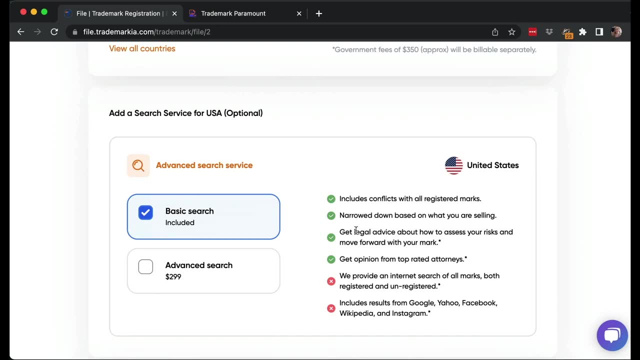 United States is $399, one class, plus the government fee. Okay, Basic searches included, including conflicts. narrow down what you're selling. get legal advice. It has a little dot, So we're going to have to look at what the dot. 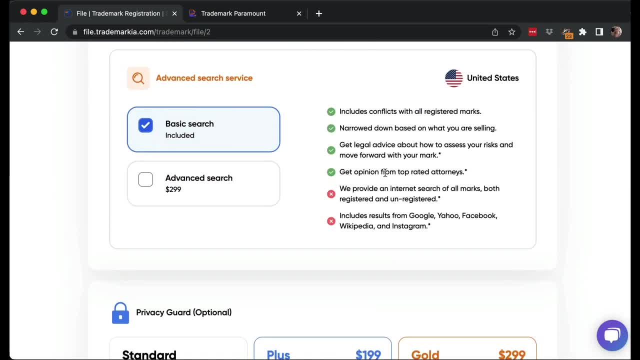 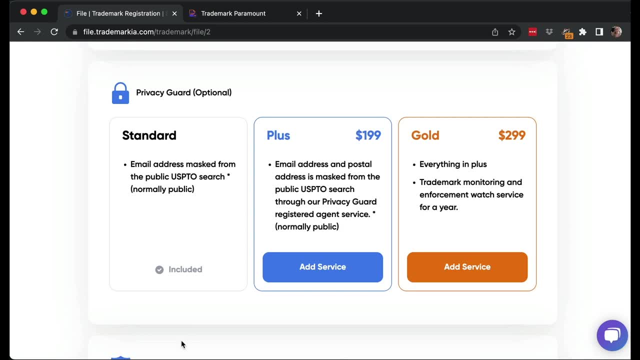 I mean I wish they would say what it was right there: Get opinions from top rate attorney. So we actually have the word attorney involved here. So there's some legal things happening, Okay. So privacy guard we do not want. oh, they have some kind of privacy or registered agent service. I 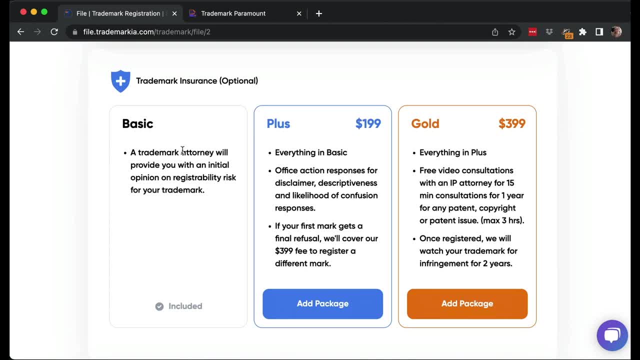 think that's a its own problem. Okay, So a trademark attorney will provide you with an initial opinion on your register, register ability, risk for your trademark And for $199,. you get office action responses for certain things: disclaimers, descriptiveness and likeliness. 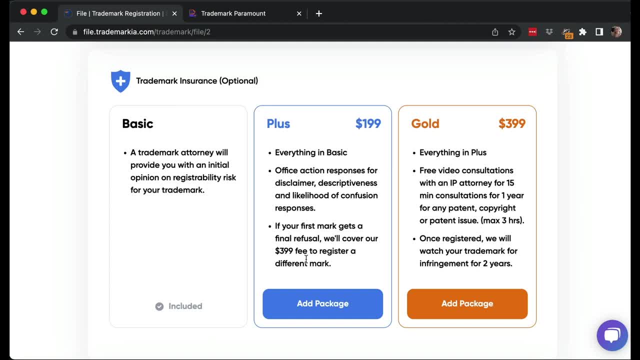 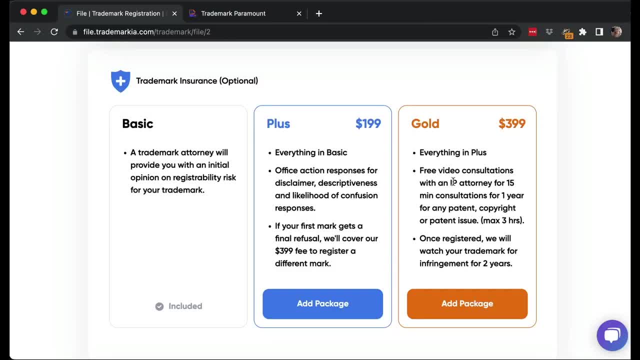 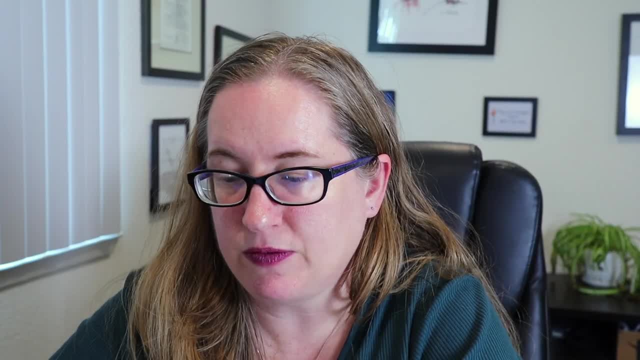 zoom was, by the way. And then the gold level. you get video consultations with the IP attorney for 15 minutes for one year for any issues, max three hours. That's actually a fair amount. That's actually a good price for that. And then, once register, watch it for two years. I'm not going. 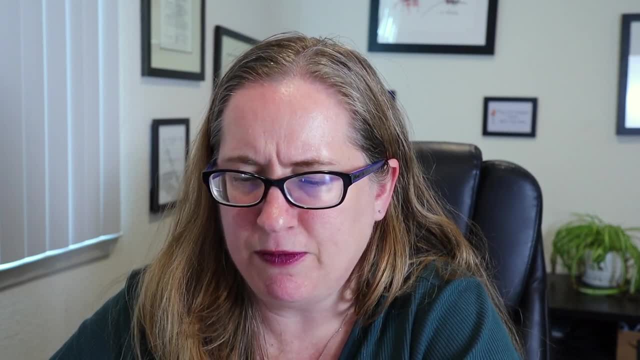 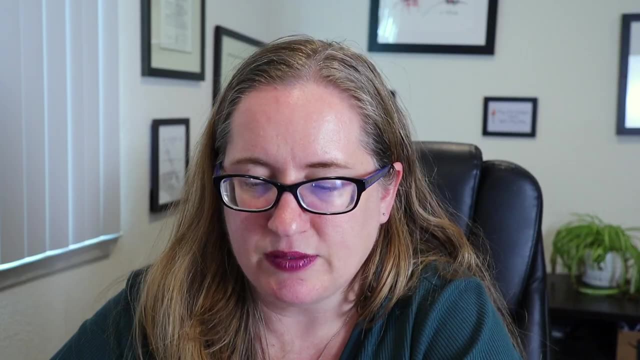 to select these, but these seem fairly reasonable. It's called trademark insurance, which I need to know is a clever little thing They're calling it, but that's not what it is. but that's fine. It's processing. You can pay more to get expedited processing standard. It might take five or six. 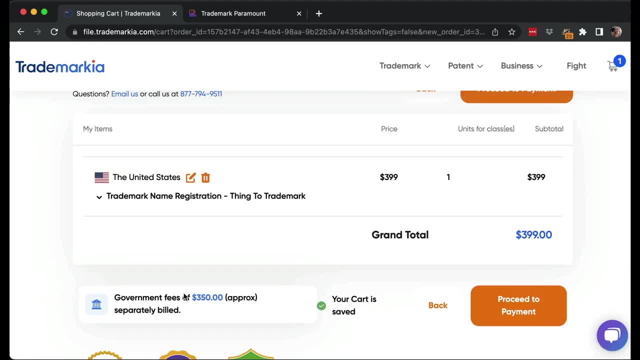 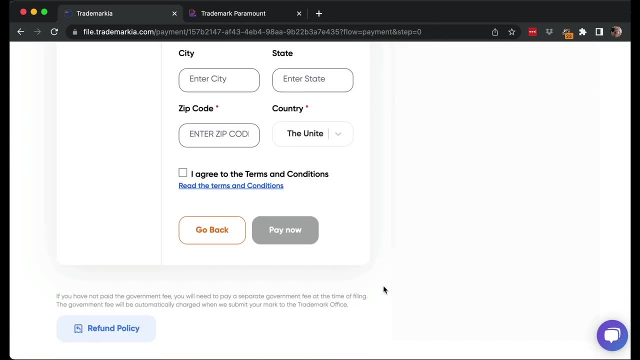 days. That's fine, We're just going to go with that. Okay, So, government fees at three: 50.. I want to see what they do about that. one. All right, Proceed to payment. Okay. So what is the terms and conditions? If you have not paid the government fee, we will need to pay a pay a. 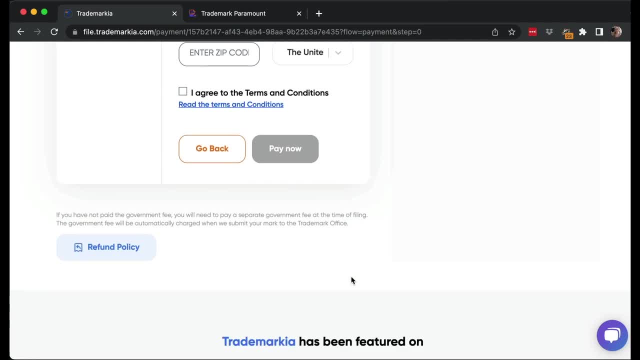 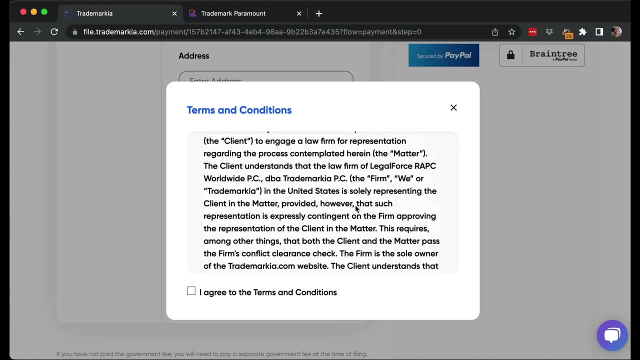 separate government fee at the time of filing. It'll be automatically charged when we submit it. All right, What's the terms and conditions? blah, blah blah. This is like very difficult to read. Okay, The law firm of legal force are a PC, worldwide PC doing business. 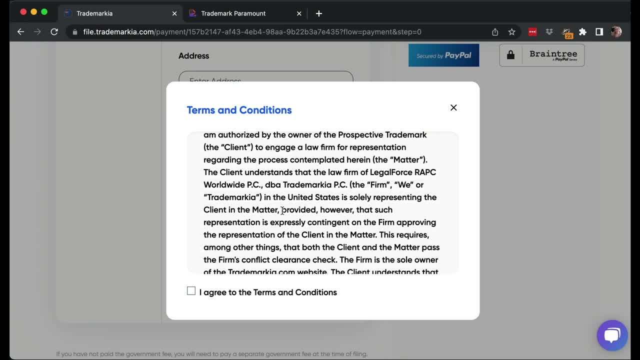 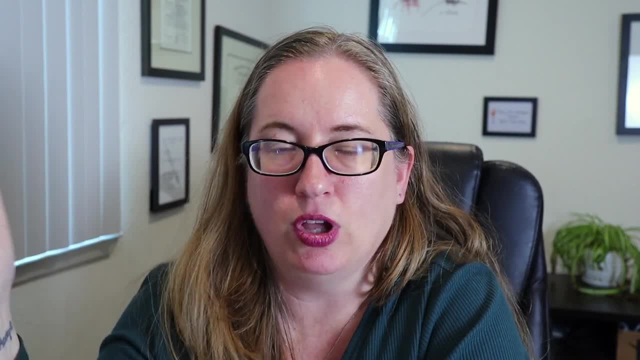 as trademark. PC is in the United States solely representing the client in the matter. So here's something that is interesting: is trademark? Yeah, It's just a DBA of a law firm. This is a law firm, So if you sign up for this, they're. 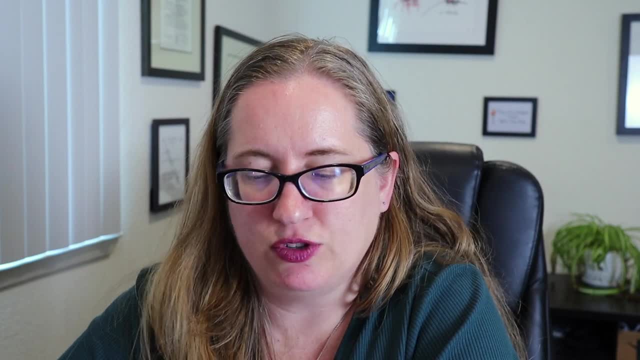 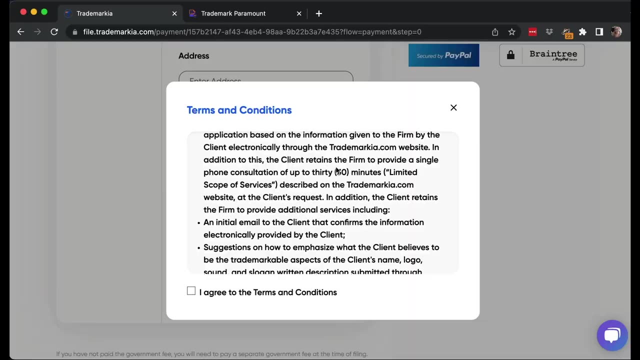 the law from representing you in this matter. Obviously, you have to do a conflict check and they could let you go If you don't pass the conflict check. For those of you who don't know, that is always true with them. When you hire a lawyer, the client will retain the firm to provide. 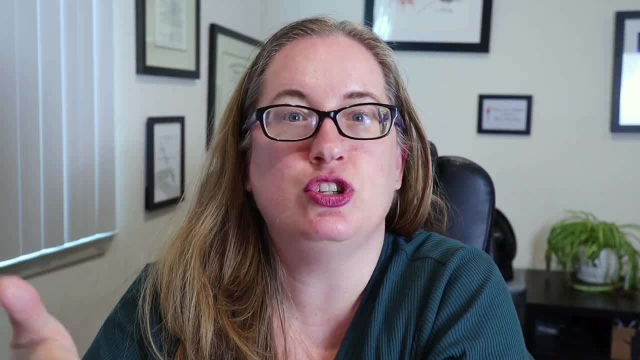 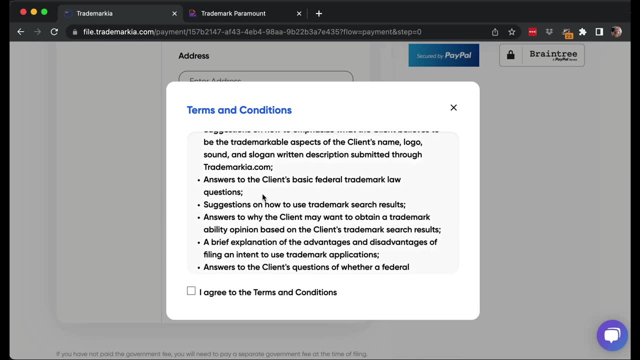 a single phone conversation of up to 30 minutes. So it's similar to legal zoom, where you get a 30 minute call included And then you'll have initial email suggestions on what to change. answers about questions. brief explanations, other answers to questions, suggestions how to proceed. 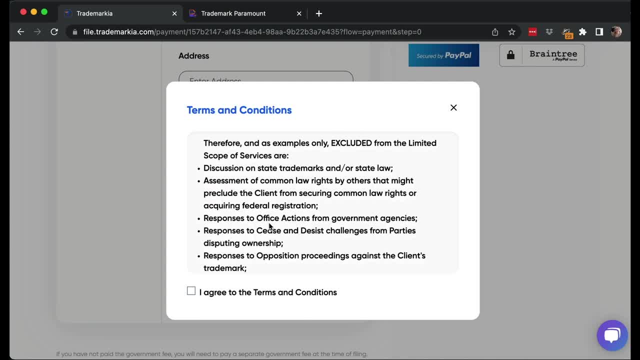 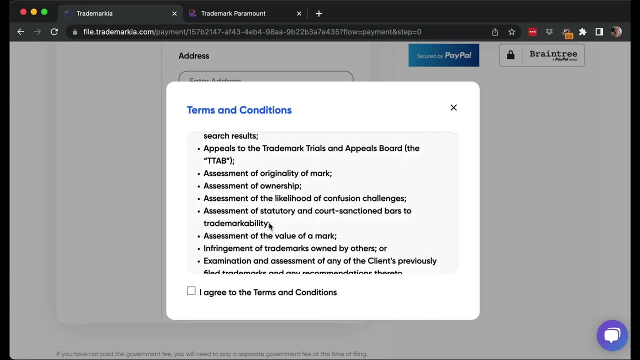 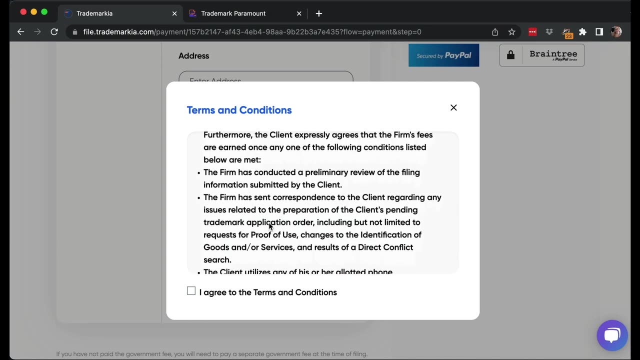 to a consultation. So things that are not included: discussion on state trademarks, common law rights, responses, office actions, cease and desist, opposition proceedings, really a whole bunch of other specific things. but you can retain them to do that. So for service fees, let's see if I had 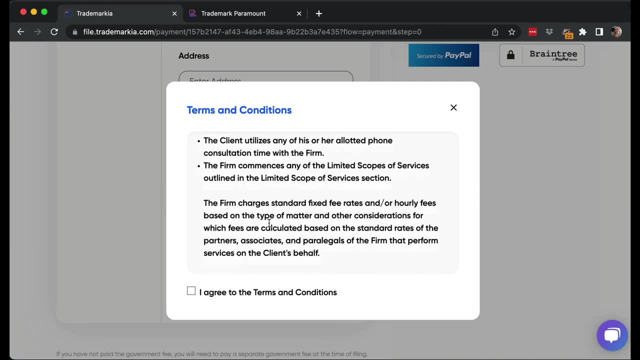 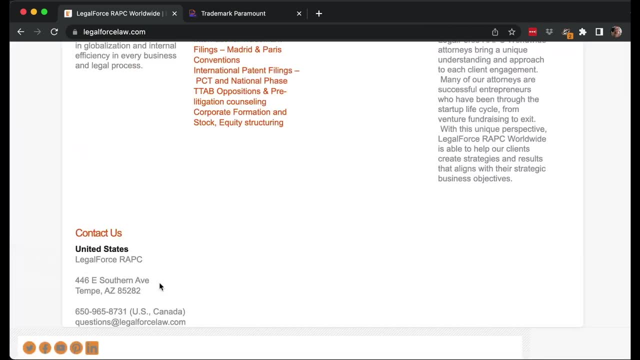 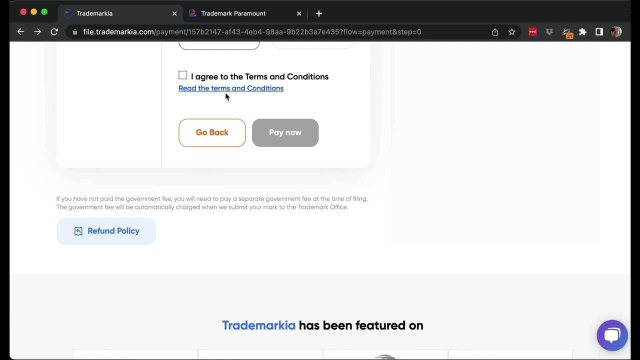 doesn't actually say what their hourly rate is. It has standard hourly rates. Let me actually click on their website and see if we can find out what their standard hourly rates are. I don't. this is it's not very good website. I don't see anything about what their fees are. So, going back to the 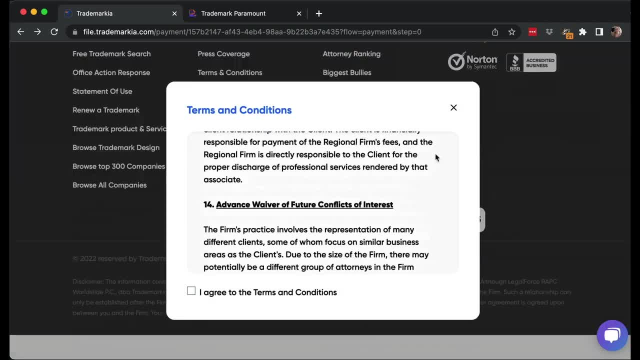 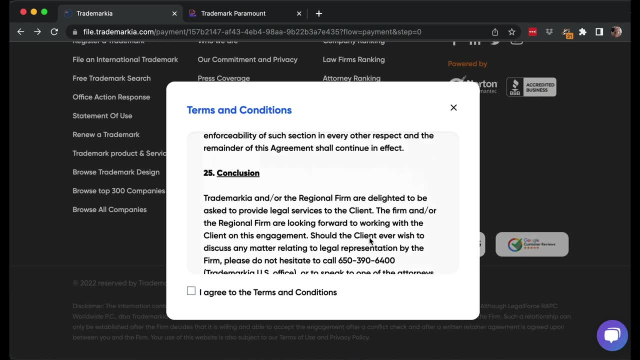 terms and conditions, which is horribly long. This is, oh, my computer's like freaking out because I'm scrolling through it. Okay, There, we have an address here. It was revised in 2021.. I'm not very happy about what the terms and conditions are and the fact that it's all buried, but I am. 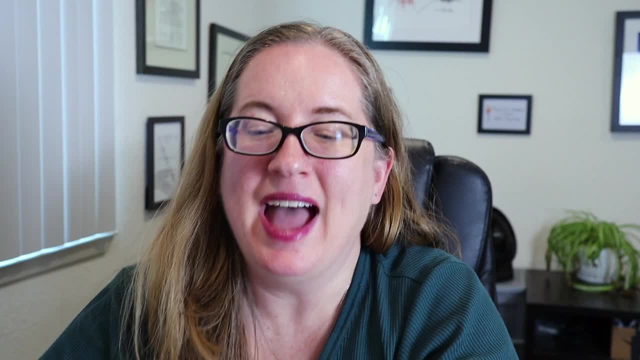 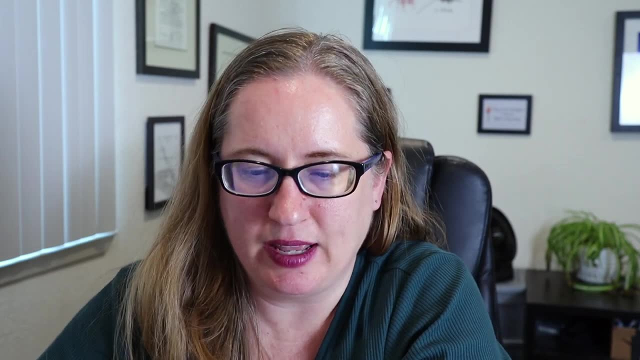 I do really like that. an actual lawyer is representing you and the law firm is involved, So that's very good. 399 seems to be a very reasonable price for what you're getting. You can pay with multiple different methods of payment. What's a refund policy You? 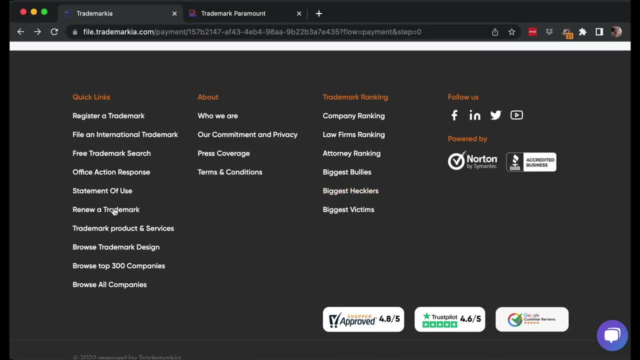 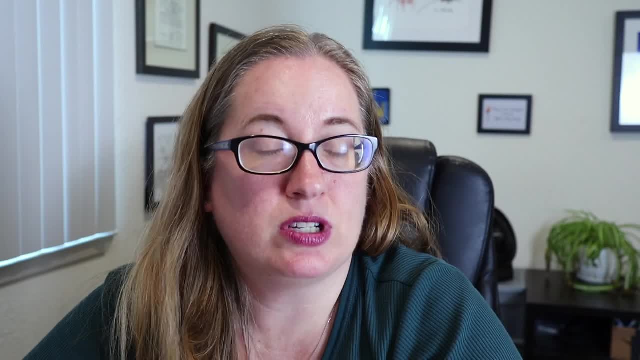 know, cause that's vague, saying whether or not you're satisfied. They also have a lot of other resources here on their website. So the last thing we're going to look at is something called trademark paramount, which advertises on YouTube, And so I wanted to see what they were and see if 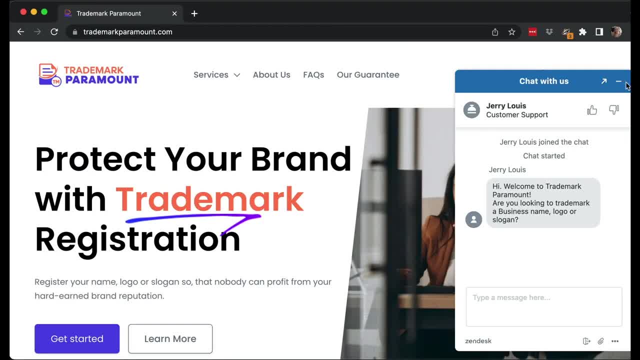 it's something that I would recommend to you. So, trademark paramount. first, they have a chat that keeps opening up over here. I'm closing that, Okay- On their website. they have a phone number over here that you can call at 855,, which is probably. 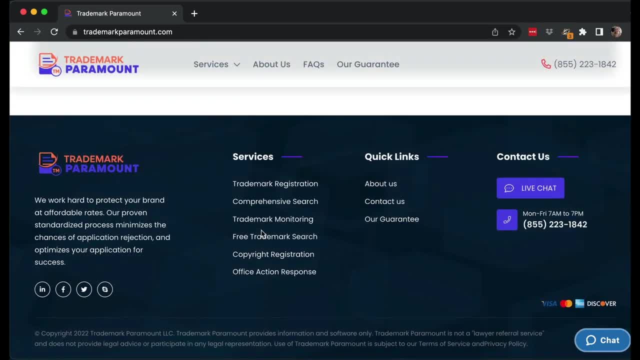 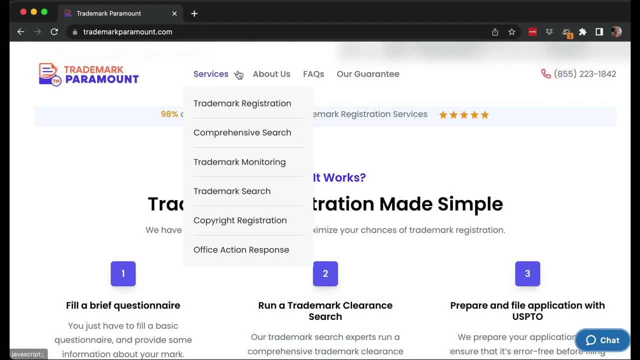 a free number And then they have their chat and yeah, no address or anything like that, But typically that's what they typically have. So they have trademark registration, They have searches, copyright registration, office action response. Those are the only things that they have. 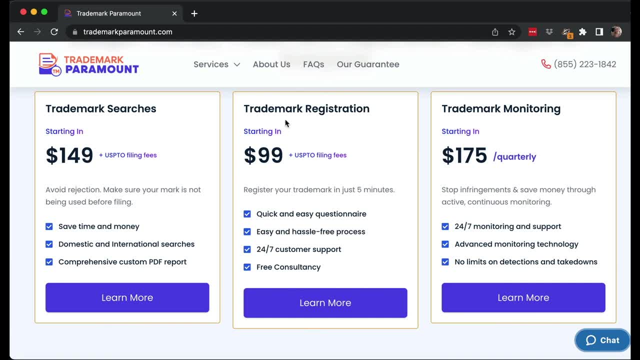 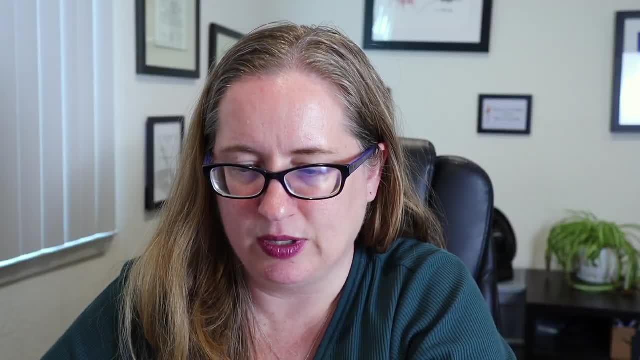 So what are their fees? All right, Searches start at 149, registration at 99, trademark mark monitoring at 175.. I'm thinking there's no lawyer here just because it's only $99.. And that seems to be the standard that if it's a lawyer. 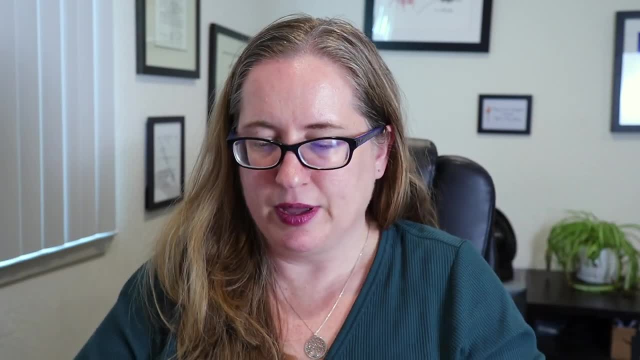 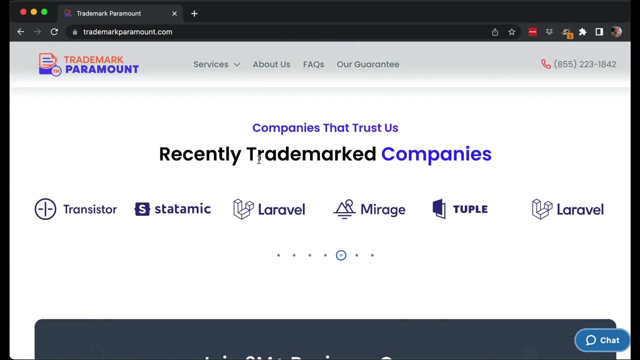 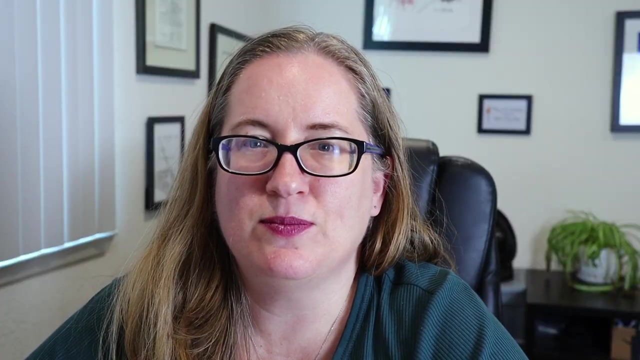 we're talking hundreds of dollars and it is no lawyer. It's $99.. So let me look at they have testimonials with just first names, So it makes me feel suspicious about something. They say they have 6 million business owners, So I am interested in. 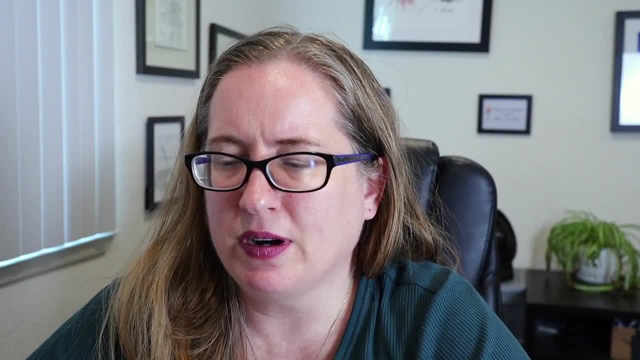 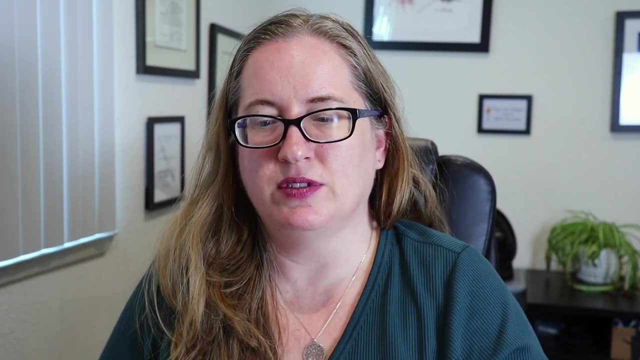 whether or not that's true, because trademark and legal zoom have hundreds of thousands of trim marks that they found And they're like the top In the numbers of how many they've done So: 6 million. where's that number coming from? 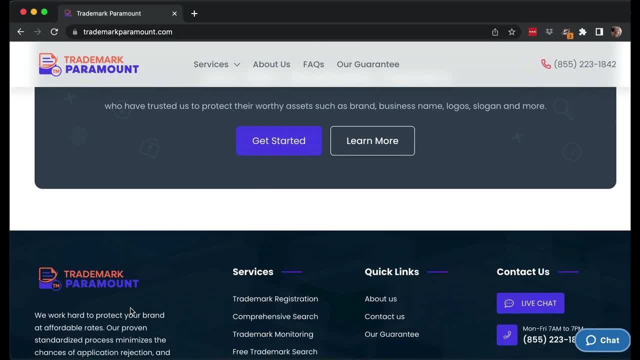 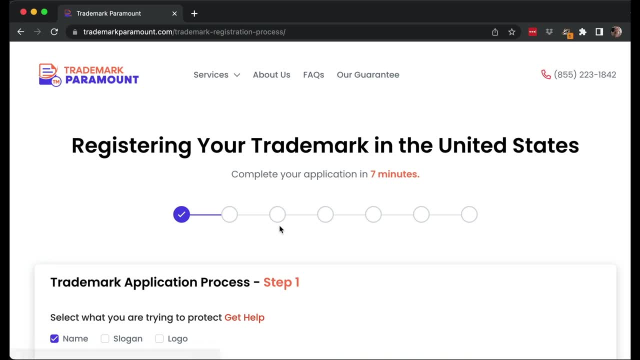 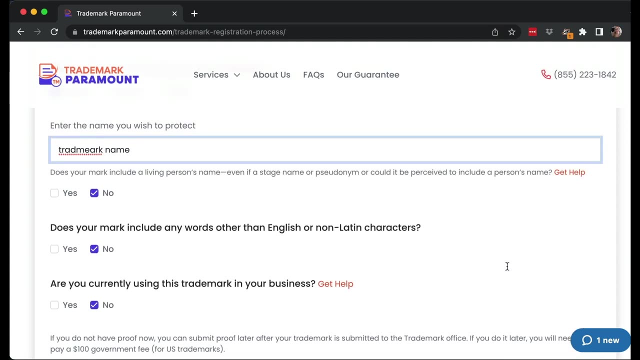 But it also says their brand, business name logo, slogan: more: Yeah, Yeah, I don't know about that, We'll, we'll see, All right. So looking at the actual trademark registration, let's just click started. What are you trying to protect Trademark name? It's not even spelled, right, Are you? 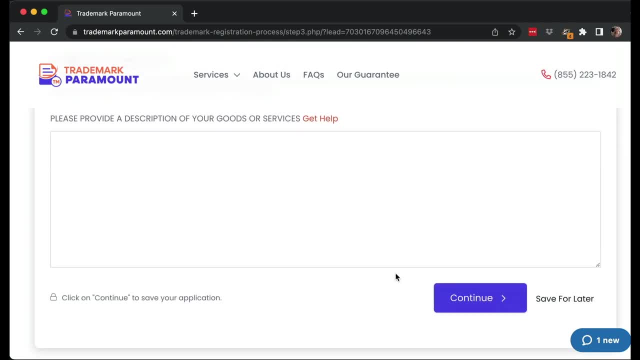 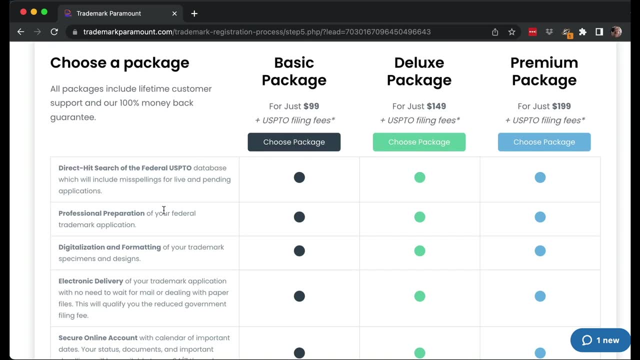 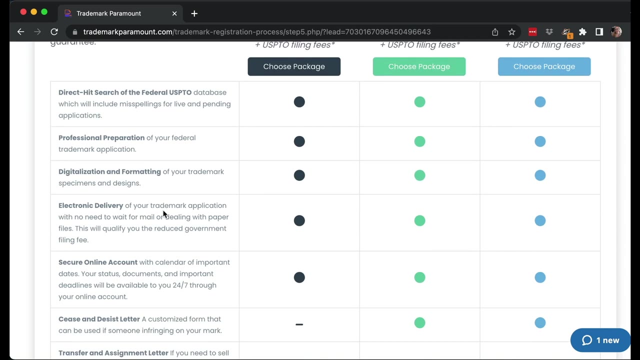 currently using. this actually looks very similar to the trademark engine. All right, Trademark classification. Okay So basic package: direct hit search, professional preparation. I think these guys just copied off the other website Digitation formatting, electronic delivery. This looks like it. 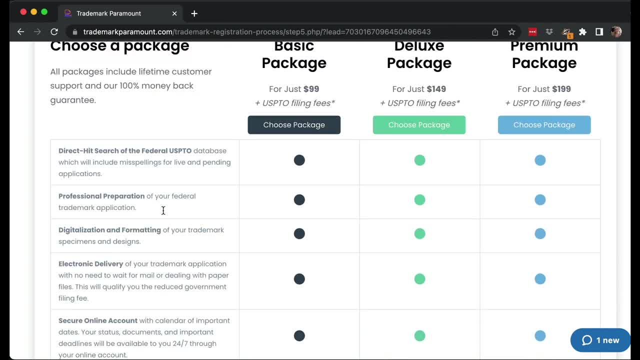 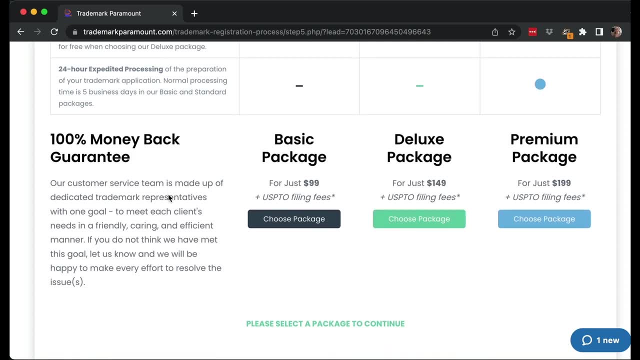 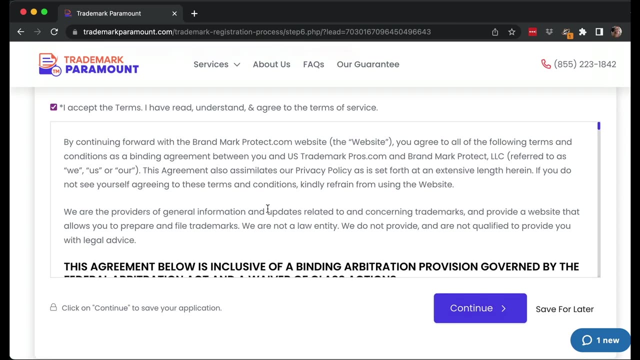 literally is copying this other website that we looked at the trademark engine. I think it might be like- I mean, they they change the font and stuff like that, but it looks like it's like literally the same. That's sketchy. Okay, Let's just pick the cheapest one. processing, Yeah I. 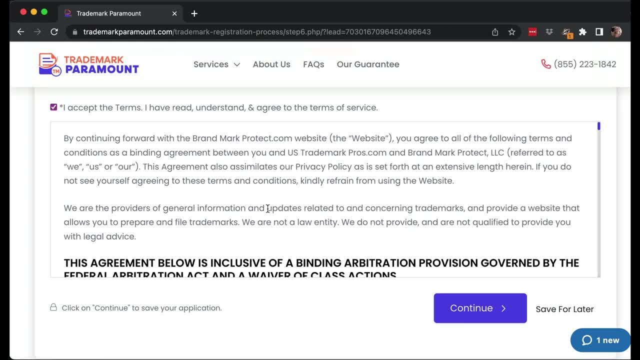 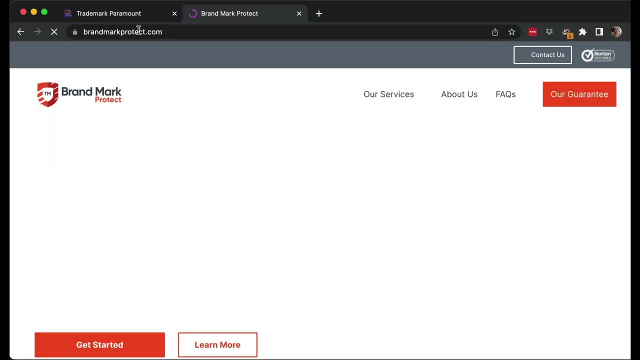 really feel like I'm continuing forward with the brand mark protectcom website, which is not this website. What is that? I'm going to put this in Google and see what this is. That's another website. I don't know about that. Are they just copying this other site? 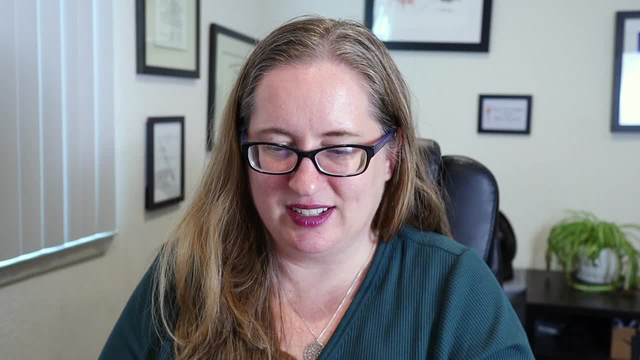 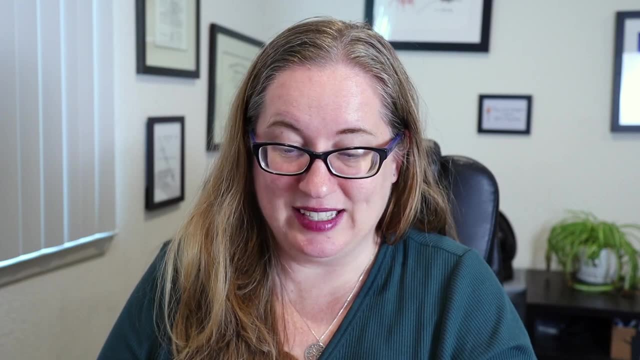 Or is that also them? I don't know. That's not good, So these guys are kind of failing my whole due diligence thing. Yeah, It looks exactly the same as the other site. Maybe they're actually the same company, right? Yeah, Oh, I'm turning on my Google. That's nuts. Yeah, There you go, I'm. 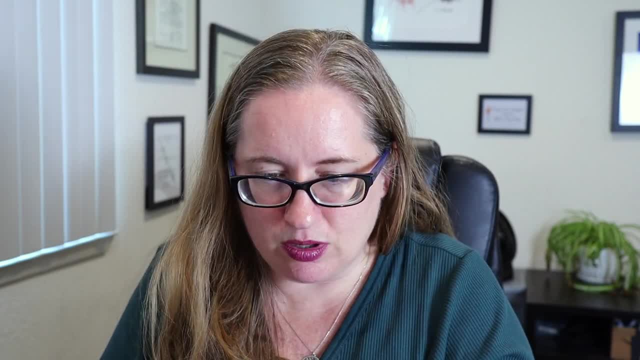 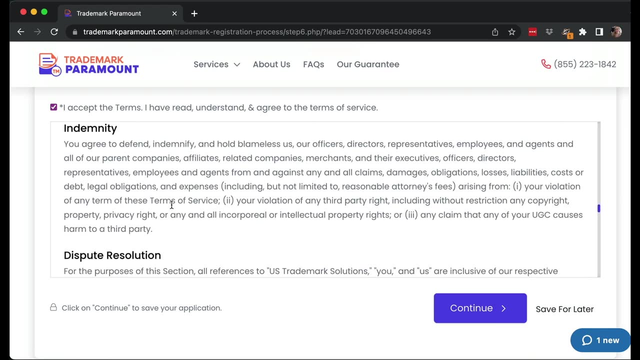 I don't know, or maybe they copied them. And then also, like the Trademark Monitoring Services, have US Trademark Pros- Who's that Who's? US Trademark Pros LLC. That's a whole other thing. So, and their arbitration, California. 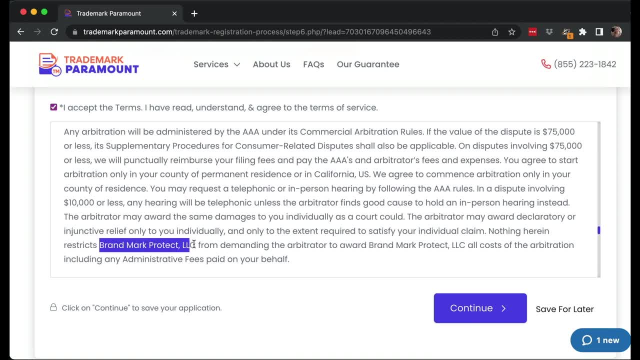 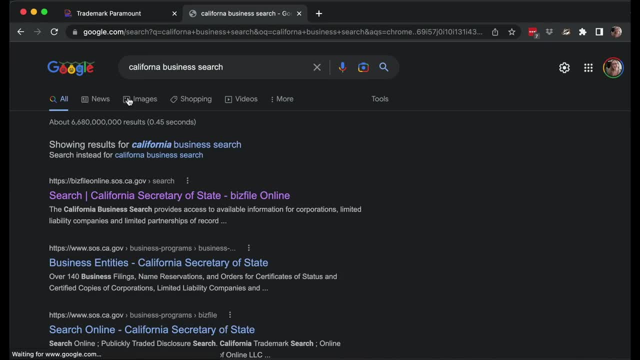 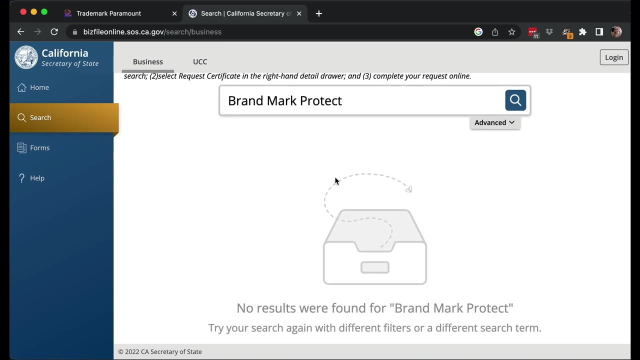 So it just says California and it says Brandmark Protect LLC. I'm actually gonna search that in California business search and see that doesn't come up as a business that exists. Let's take the comma out. Yeah, that doesn't come up as a business in California. 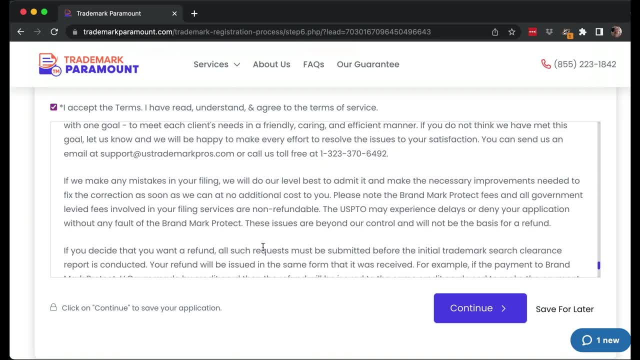 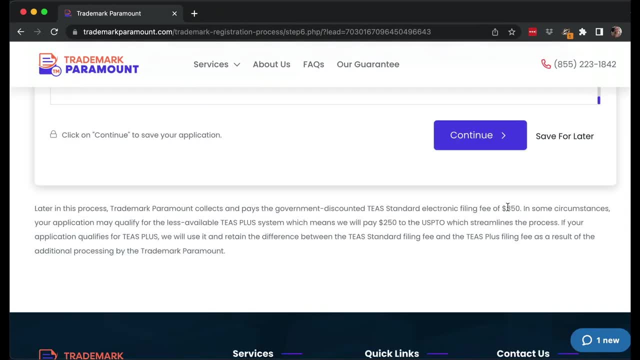 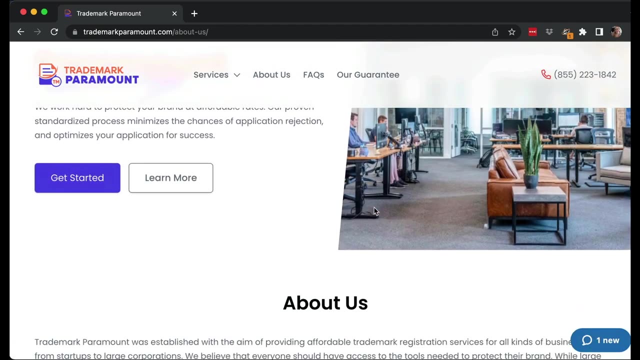 So I don't know about that 323 phone number, which is LA. Okay, later they pay the 350, and then we'll retain the difference, just like the other website did. Yeah, this is about us Gets no information really. 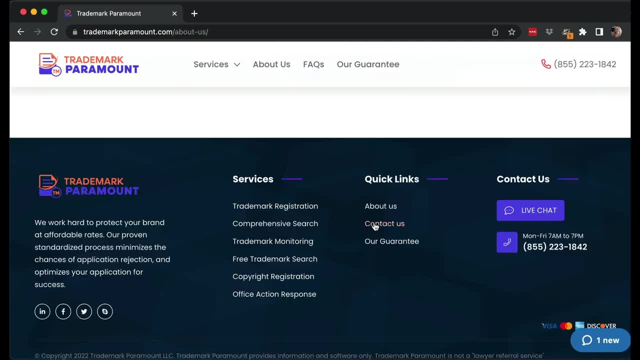 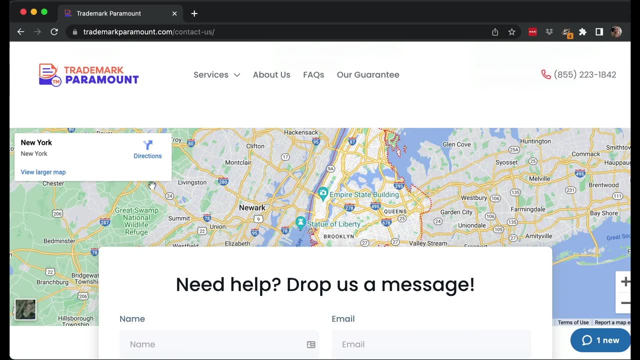 but it is, although we are not a law firm. So this is definitely not a law firm. Contact us has live chat, And then they have a map of New York. Like, what does New York have to do with anything? Trademark Paramount LLC. 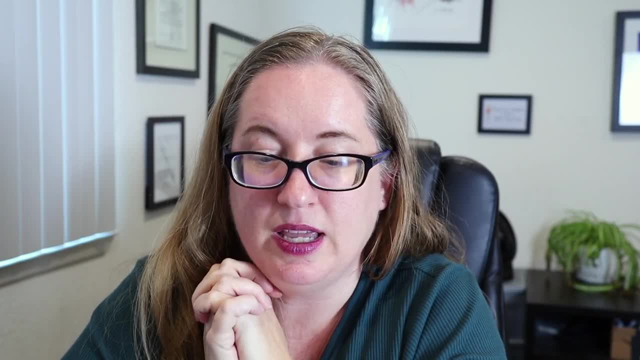 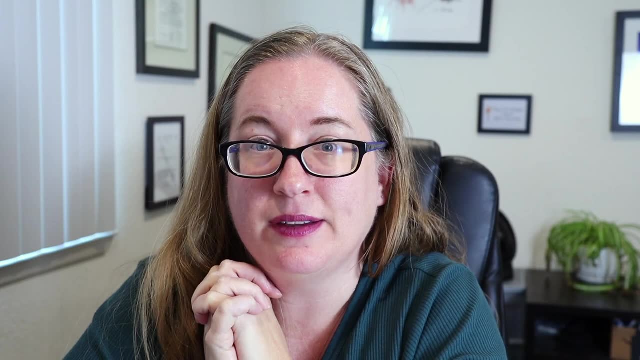 Okay, so do not hire these guys. Trademark Paramount LLC. Trademark Paramount. whoever these people are, I actually don't know. I think that they may have scraped all this stuff from other people and un-copied it without putting their own information in there. 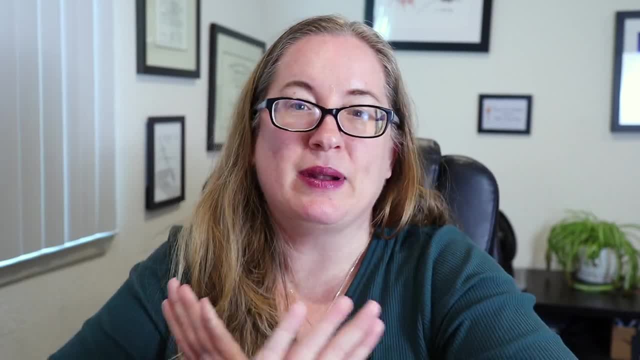 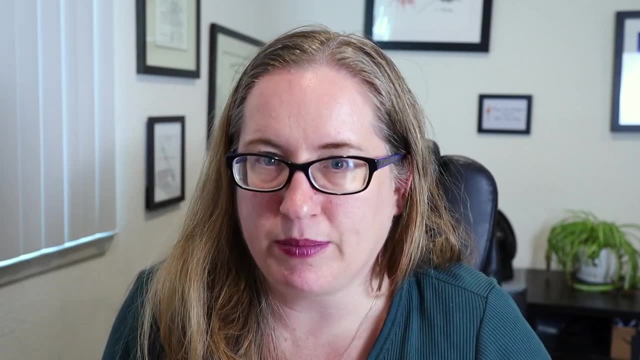 I don't even know if these guys really exist. So No, Trademark Paramount is a no, So that's simple. So, generally speaking, if you are not comfortable filing your own trademark application, you really have a couple of different options. 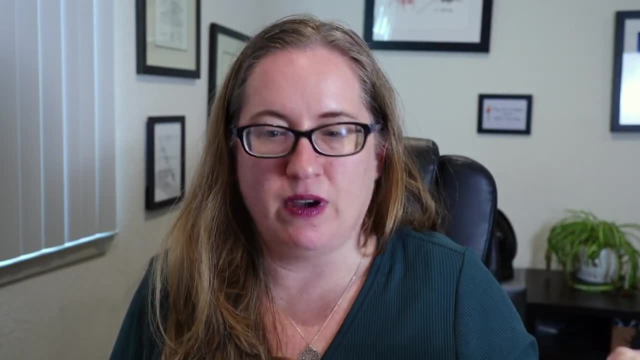 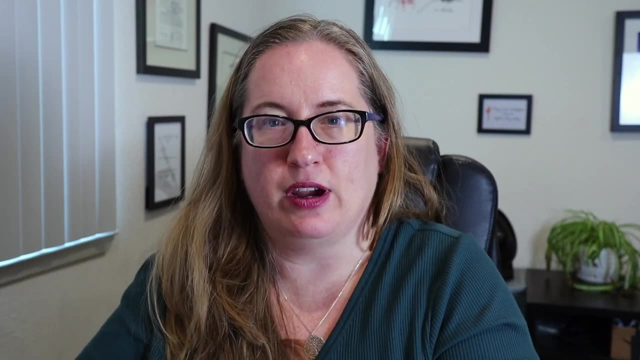 One is to hire a service that is just a service, no lawyers involved. That's the $99 kind of version of things. The next is to hire a service that has lawyers there. So that is LegalZoom Trademarkia. There's probably other ones that exist too. 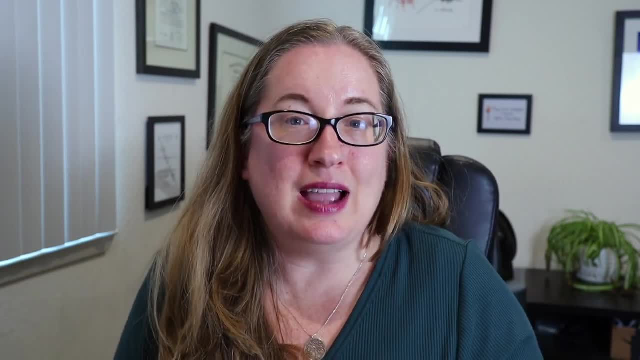 And then the top one is to actually hire a lawyer If you're outside the United States. you know, if you do not reside in the United States, you have to have a lawyer on your application. Why is that? It's just a rule. 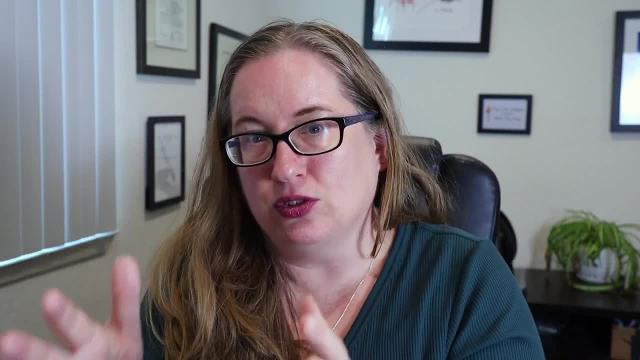 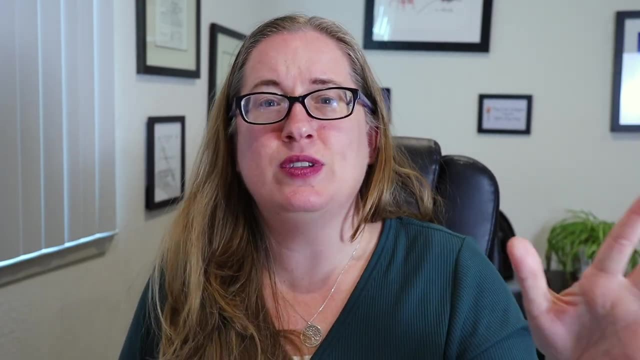 I don't know why I'm not in charge of that. So you have to use a service that has lawyers there or hire a lawyer outright. If you're just not comfortable filing it, should you just do the kind of $99 thing? I do not recommend doing the kind of $99 service only. 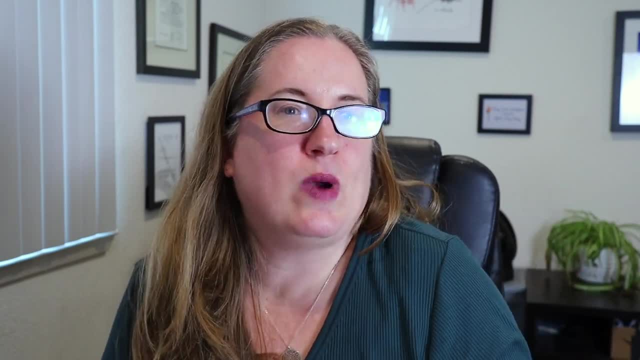 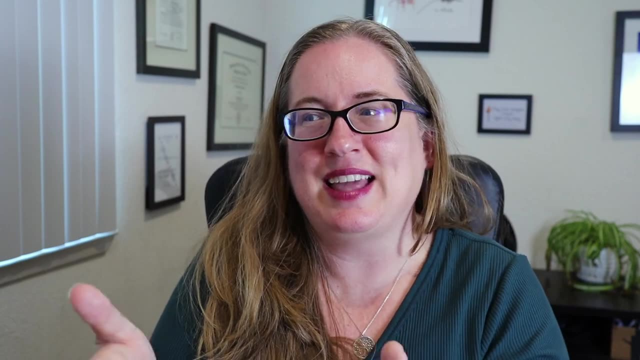 because I don't really see what they're doing for you. You're actually having to write your own class anyway, and you probably don't even know how to do that, So without watching one of my videos or something like that, and then you could just do it yourself, right? 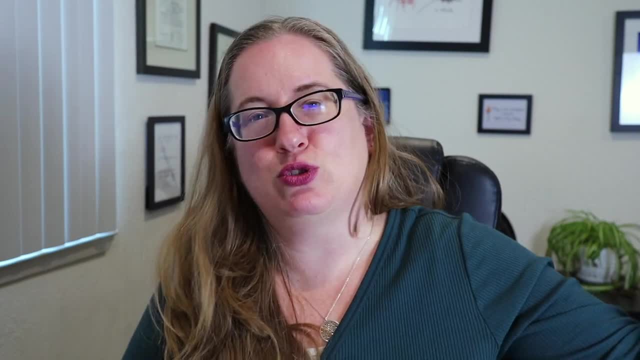 Like I don't really see what you're getting. And then you're going to be in their subscription thing and all these subscriptions, and I'm not really a big fan of that. So I would say, if you're really not comfortable doing it, 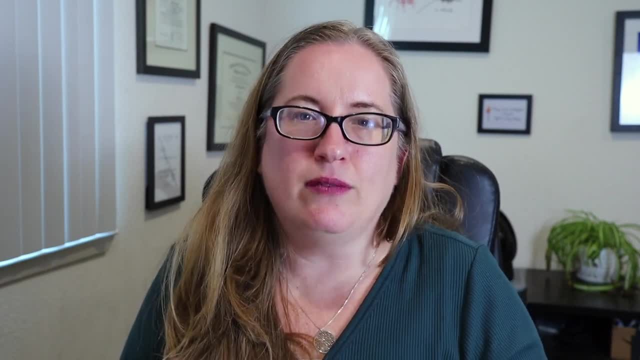 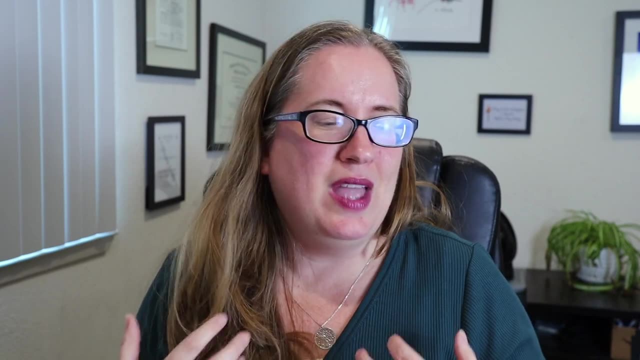 you want to have a lawyer in some way, shape or form, And so I'd either have one of these services or hire your own lawyer that you have a direct relationship with, And if you're picking between Trademarkia and LegalZoom, 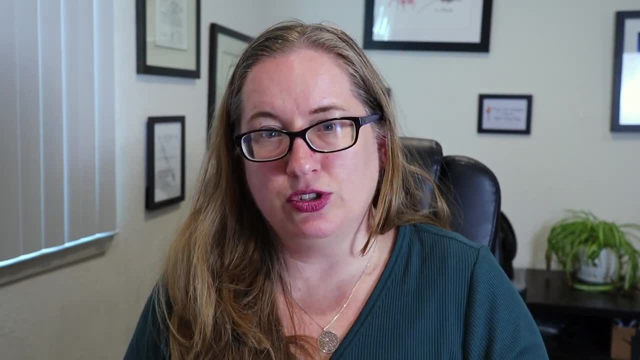 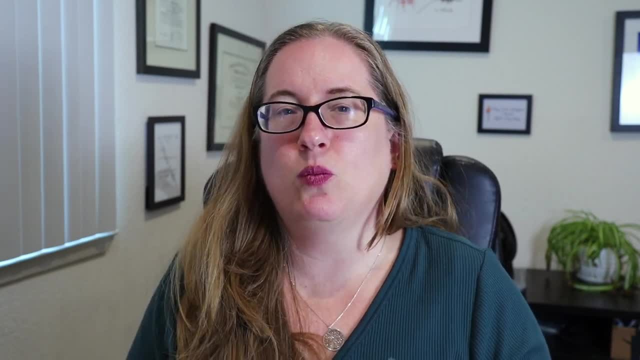 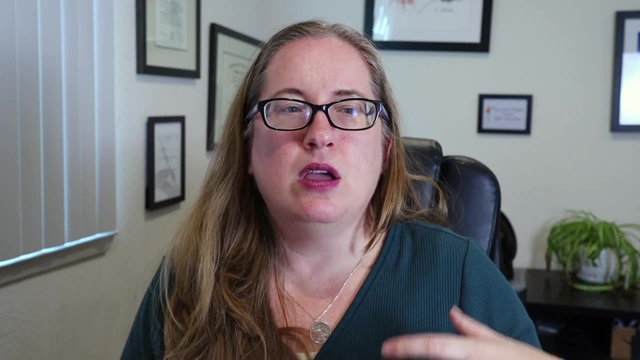 I've had. so many people have bad experiences with LegalZoom, While I haven't heard about that with Trademarkia. I'm not saying it doesn't happen, but I haven't heard about that. I also really liked the fact that Trademarkia 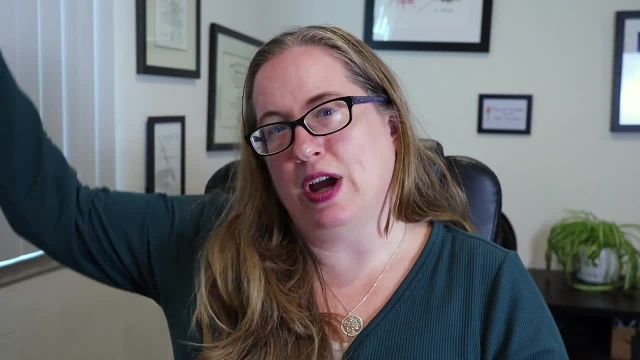 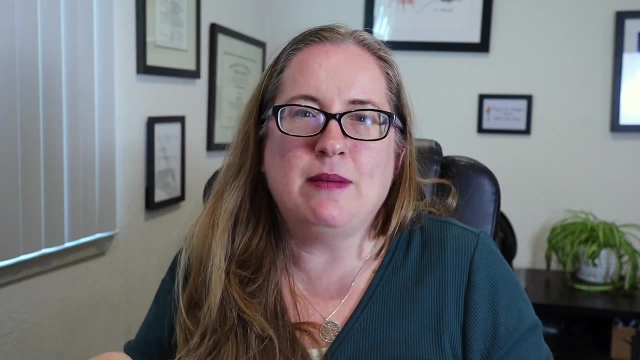 is just the DBA of the law firm, where LegalZoom is a big, huge, giant company that has a whole bunch of parts to it And then you're getting in the lawyer over there. Like I think it may make sense to be more direct. 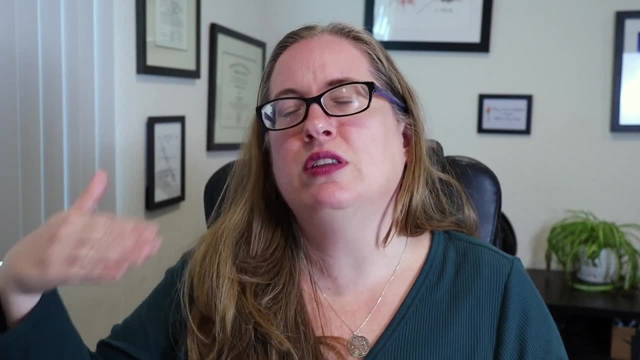 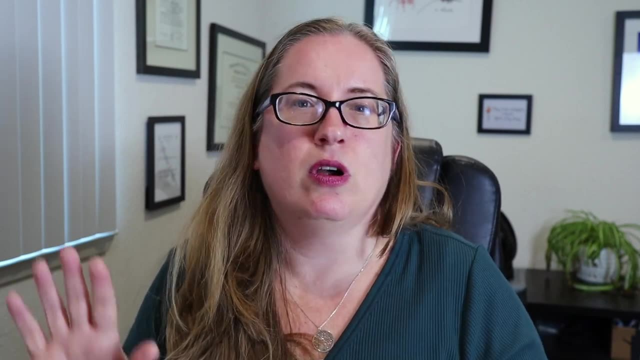 with the lawyer, and also their fees are a bit lower. LegalZoom seems to be putting their fees higher and higher recently, And so if it was up to me, I would say Trademarkia over LegalZoom, And then, of course, if you have a really complex situation, 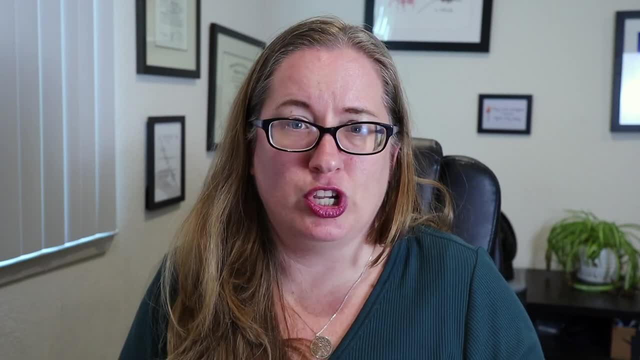 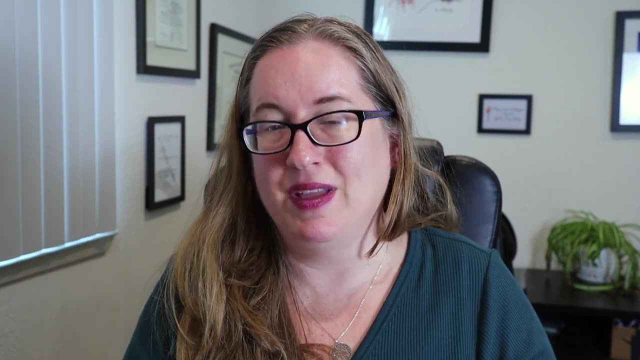 you may want to hire your own lawyer outright, especially if people are already infringing you. Now, side note: if you're getting a trademark just for the Amazon Brand Registry program, you may actually want to go through that program and use the lawyers that they have relationships with. 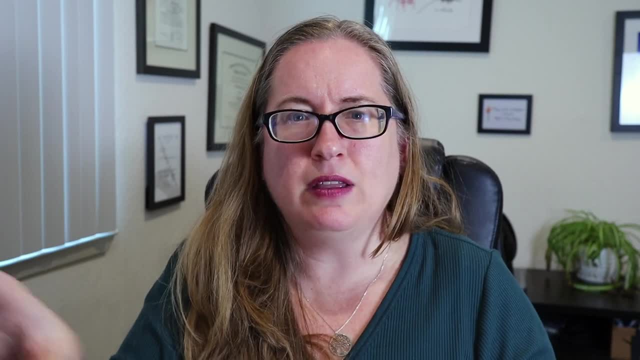 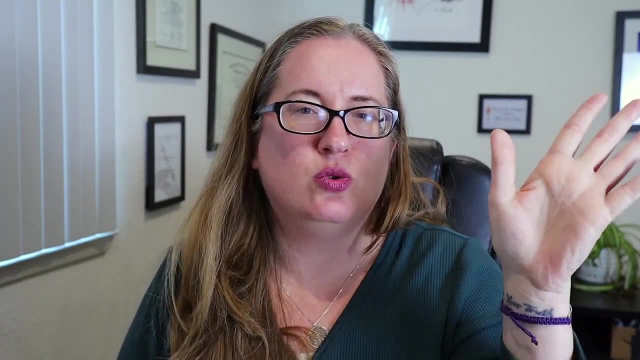 because the fees will be comparable to these other filing services And you're kind of in the Amazon Brand Registry program. I actually did a video like that. I'll link to it too, so you can check that video out. Thanks a lot for watching. 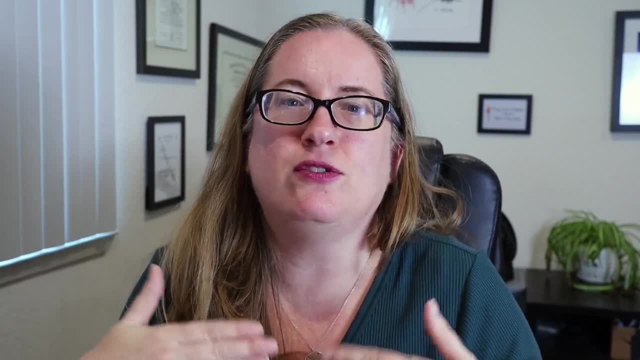 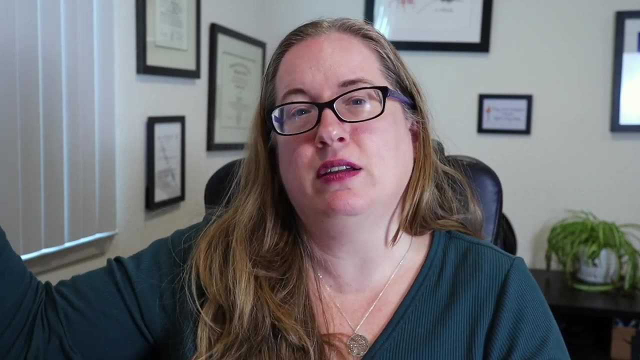 This has probably been a ton of information, but I wanted to give you some ideas that if you're not comfortable filing a trademark for yourself, where you could get more help as opposed to just filing, you know, hiring a lawyer- If you had the fees for that, you could go do that. 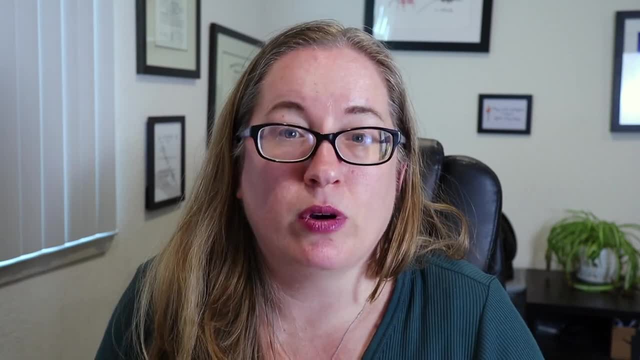 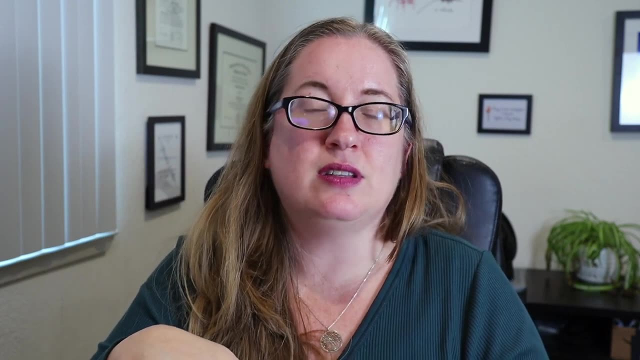 But what are other services available that may be more affordable for you? If you found this video helpful, hit the thumbs up button- subscribe. if you'd like more videos like this, Leave a comment below if you have any questions of something that we talked about in this video. 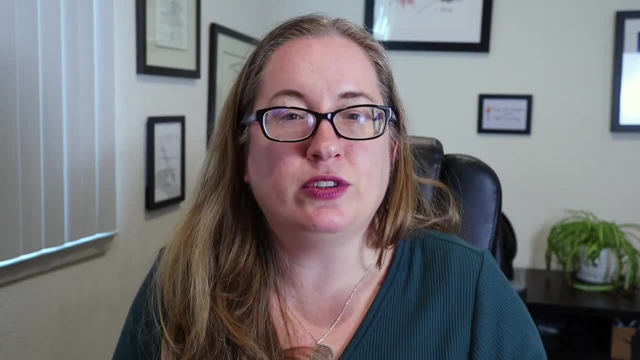 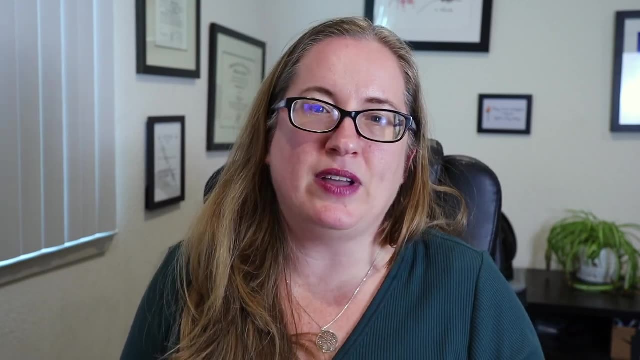 and I'll try to point you in the right direction. If you'd like to support the channel in making more videos like this, you can sign up for the Patreon. You can join the free Discord. You'll learn all about that stuff in the description below. Thanks a lot for watching. Bye.